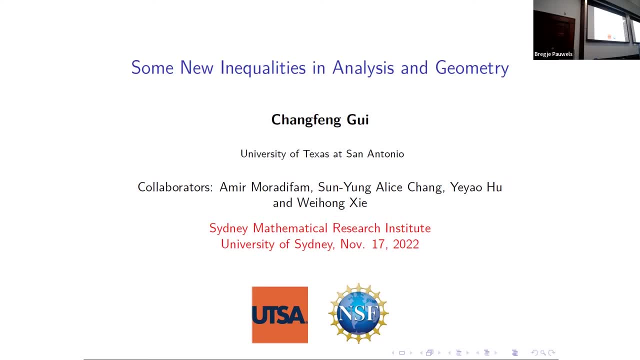 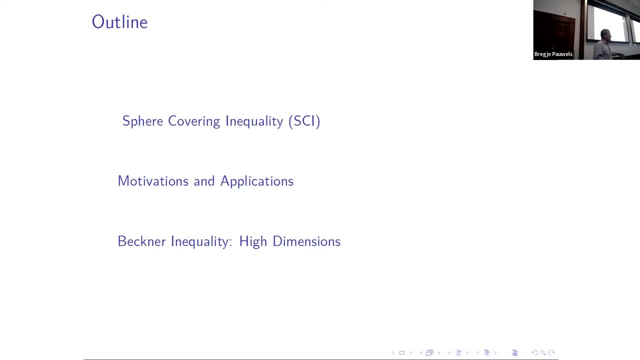 postdocs and students, and they are now in Central or South University of China. So I will first explain The new inequality, called the steel covering inequality, which we discovered and proved a few years ago, and we explained the motivation and its applications. 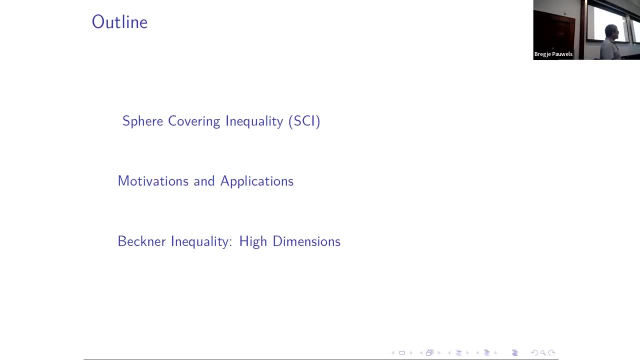 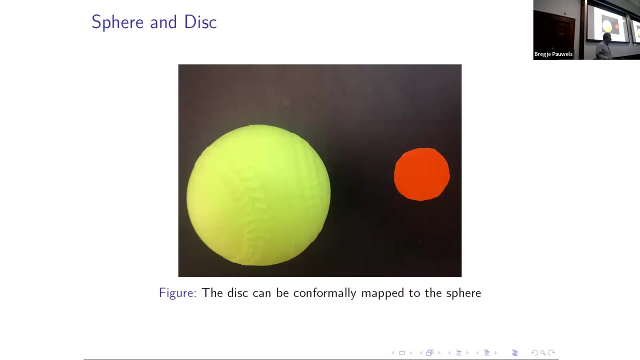 Then we'll talk about higher dimensional inequalities, like Beckman inequality, and it's basically a very open area and a lot of unanswered questions and results in this direction. And so here we have a ball and we have also glass rubber, flat rubber, like a disc. 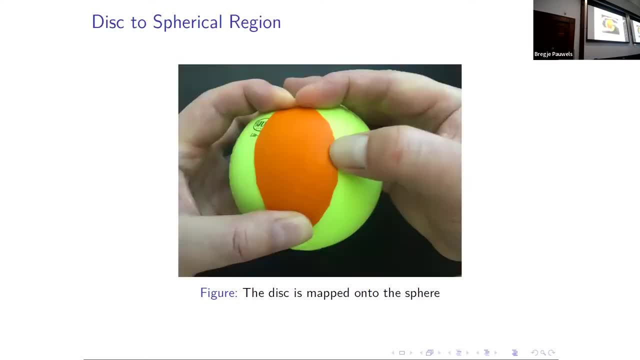 We know that we can stretch the flat rubber disc and put it on the surface of the ball. We can stretch and shrink and then put the disc on the top of the ball, exactly on the surface of the ball, without no gap between. So this is just a transformation right mathematically. 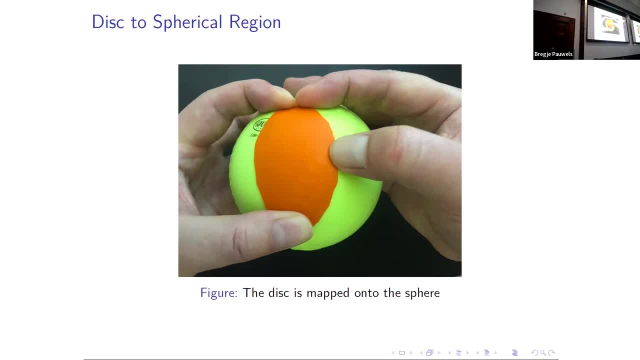 which transforms the disk in the Euclidean space to the surface of a unit ball. And of course we can do it in other, more restrictive ways: that they stretch or shrink at every point at the same rate in all directions. Of course this kind of mapping is harder to do. 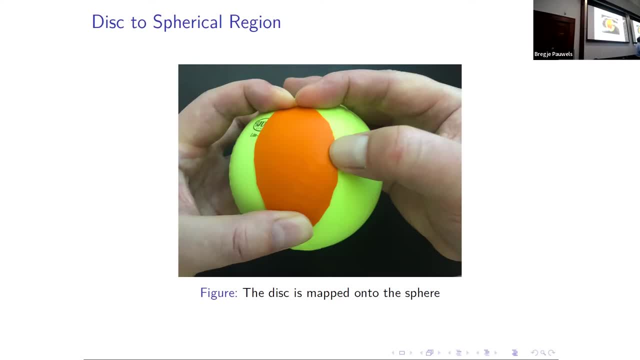 but it's doable. There are many such mappings And mathematically we call them conformal mapping. So we have many ways of mapping this: a disk on Euclidean space to sphere and conformally. Well, there are ways which make the mapping. 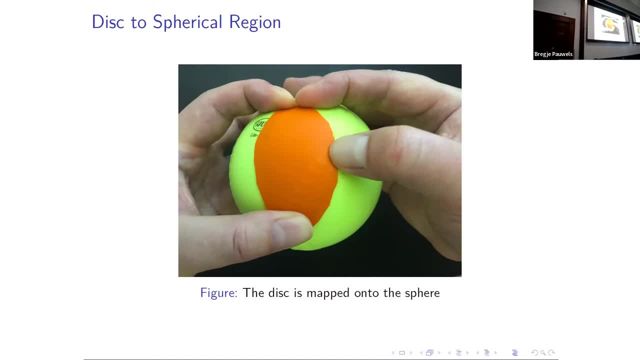 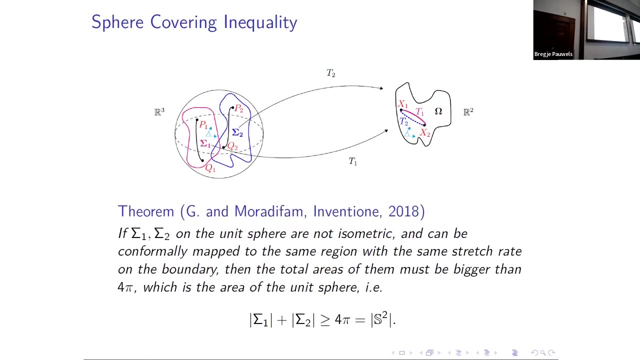 has small area on the sphere. There are also ways to make it have bigger area on the sphere by stretching more right. So, but I I want to explain a scenario. We have two such mapping, So we so this could be general flat rubber. 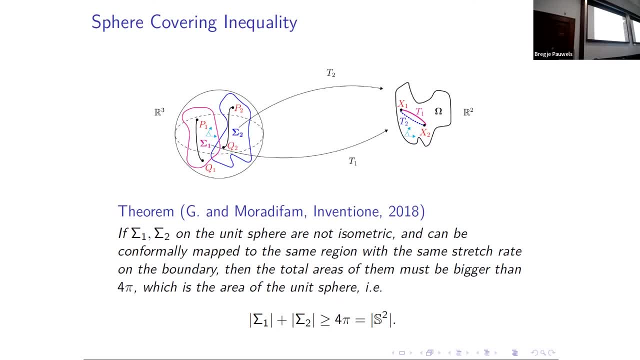 So we stretch it on the sphere. So get a region, say P1, sigma 1,, conformally, you know, as I said, stretch it in a way that at every point you have the same rate on every direction, By different point of have different rate possibly. 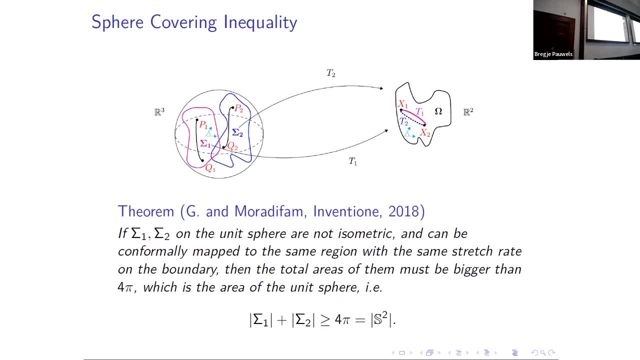 So we have, then, this area of this sigma 1,, as I said, could be small, could be big, depends on how much you stretch it, And the area could be very close to zero if you actually shrink it a lot. But now, as I said, we have another transformation. 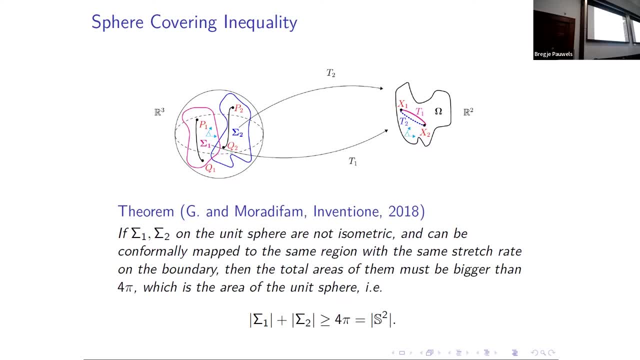 or mapping of the same flat rubber disk or flat rubber to another patch of the surface, again conformally. Now I want: these two are different. These two patches are different means they are not asymmetric to each other. They're not symmetrical to each other. 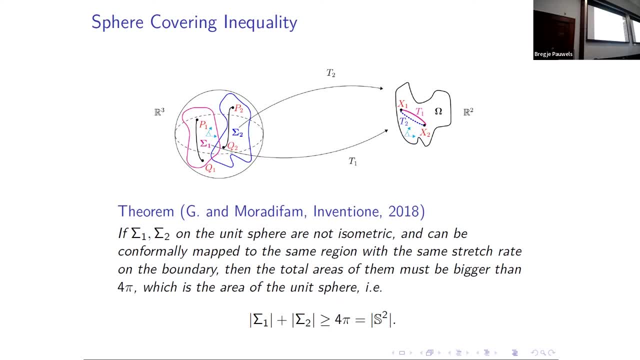 They're not just rotating or, you know, shifting. And another condition: that these two mapping has the same stretching rate on the boundary. Okay, In interior you can stretch in whatever way you like, but have to be the same stretching rate at the boundary for these two patches. 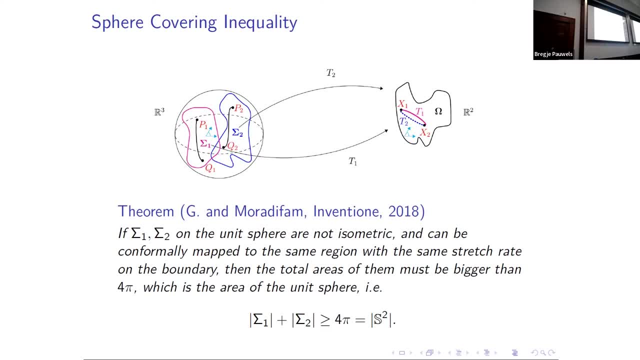 Then now I say if this happens, then I have to have the same stretching rate as the boundary for these two patches. So if this happens there will be a lot of restriction. Importantly, we say that the area of these two patches 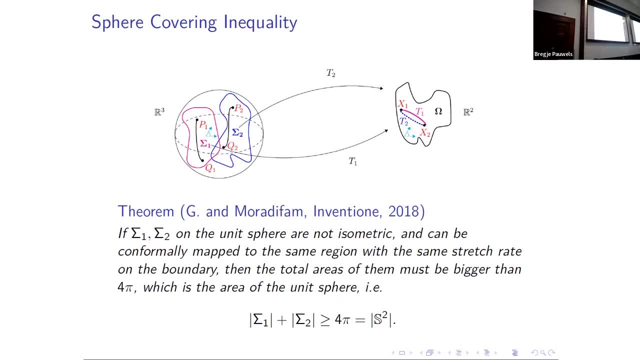 added together cannot be small. They have to be bigger than four pi. Four pi is the area of the whole sphere, or unit sphere. All right, So now we would have it could be a little bit bigger than four pi. That's what we're saying. 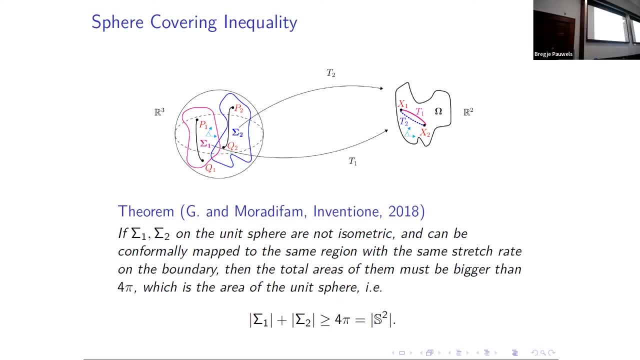 So if we have two patches then we have to have the same stretching rate. So the more, the more distance between one of the two patches and then one of the two patches, then it should be a lot smaller. What we do is to measure the rising. 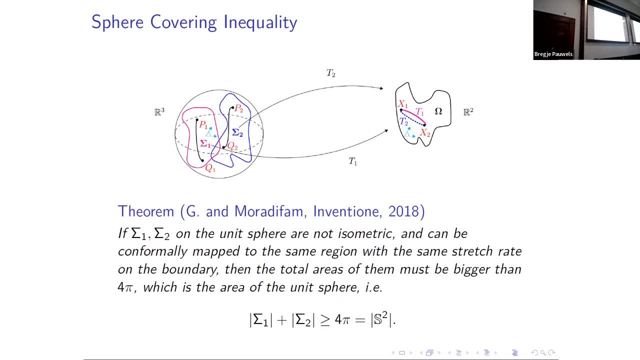 and the rising is the raising, The rising is the maximum and the rising is the maximum. So we just say we have the same stretching rate of each of those three patches, Entirely the same stretch when the of the same rubble disk. 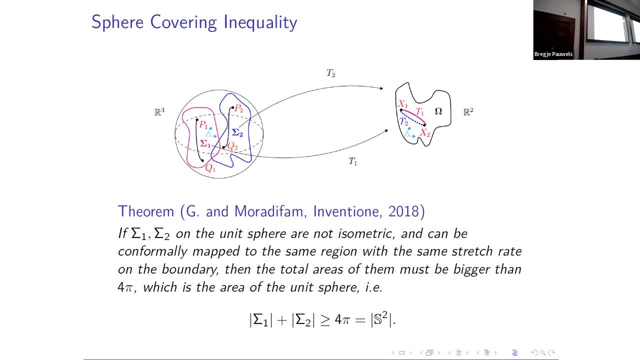 then there's a rigidity here, So the area has to be bigger than the minimum area four pi. So in other words, this area, if you imagine, arrange it area wise, it will be covered the whole sphere. So that's why we call it sphere covering inequality. 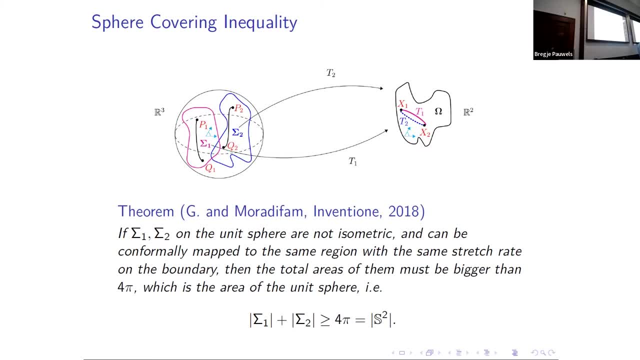 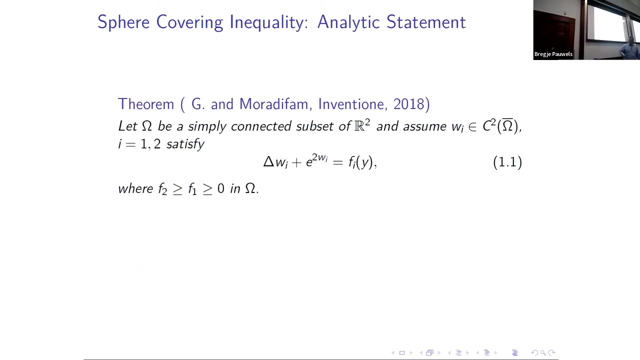 So this seems to be a very elementary, well inequality involving very elementary geometry, but things are. this is really a new inequality And, more importantly, we have many applications of such inequality. So this is the geometric way of describing the sphere covering inequality. 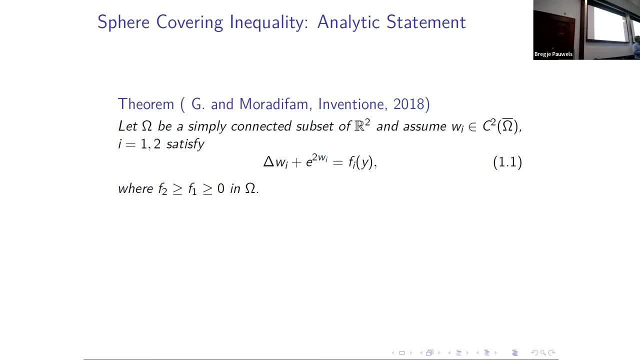 Indeed, we can explain it in a more, in an analytical way or in the flavor of PDEs. So, if you have two solutions to partial definition equation like this, so the last one is the partial definition equation, So the last one is the partial definition equation. 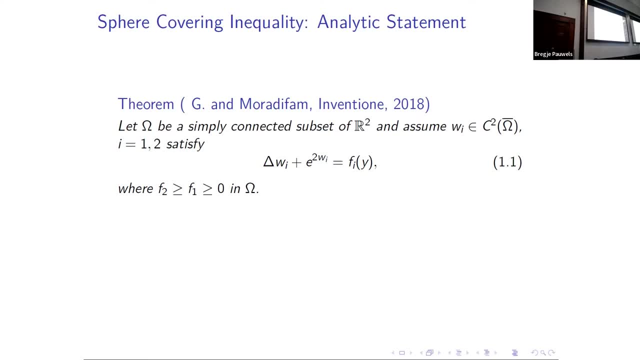 So the left-hand side is the fixed. it's not partial: U plus E to the two U, So it's a nonlinear and this type of equation we call it the Nouveau equation. The right-hand side could be homogeneous, could be zero. 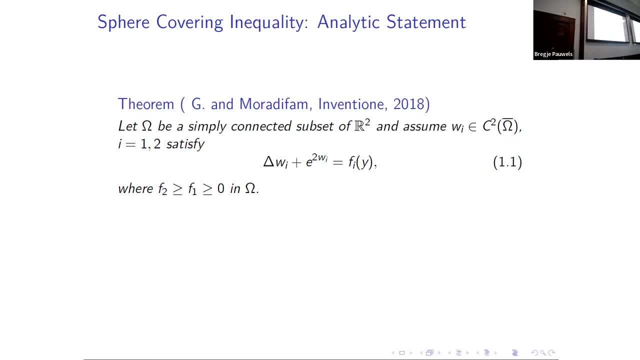 But if you have two solutions, this F2, F2, one- suppose the F2 is bigger than or equal to one, bigger than or equal to F1. And they're both positive, not negative. And then this and also the solution: 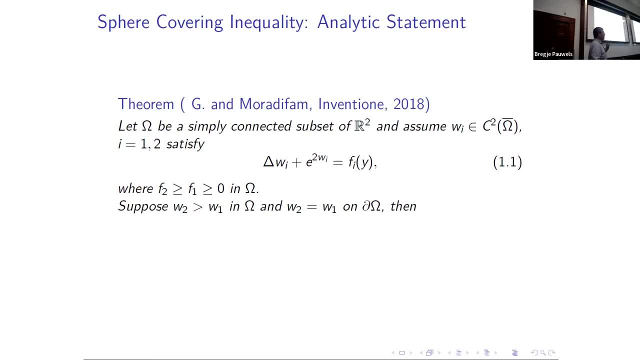 the W2 is bigger than W1 in the interior of the domain, but they are equal on the boundary of the domain. Then we say: the integral of this two sum will be bigger than equal to four pi. Of course, the connection of geometric integration. 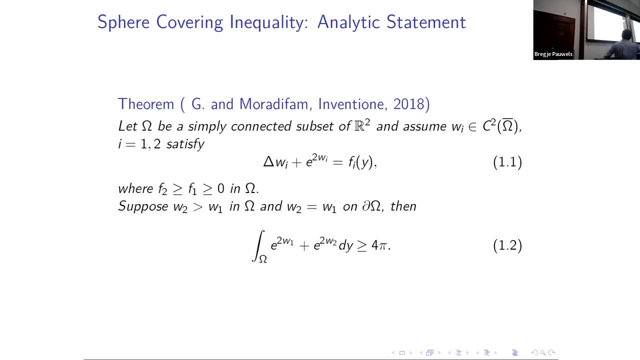 for example. So the geometric version and the analytic version is that this e to the 2w1 is the conformal factor of the surface associated with the patch And this, so each term is, really means area geometrically In general, we can have this surface be more general surface, not just sphere. 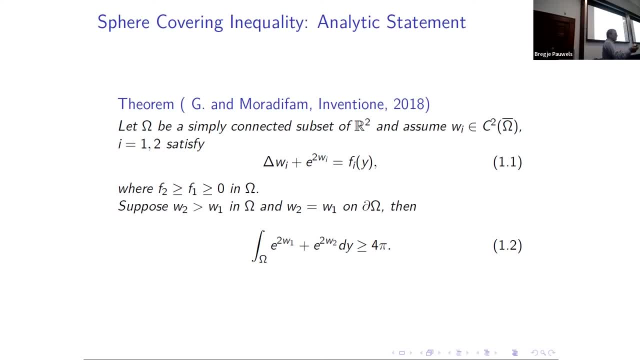 And we could also have surface with different mapping on different surface and as long as the certain sort of relation between surfaces. But anyway, this is an analytical version of the sphere covering quality, saying that they are integral of two terms, At least have a lower bound for solutions of two equations. 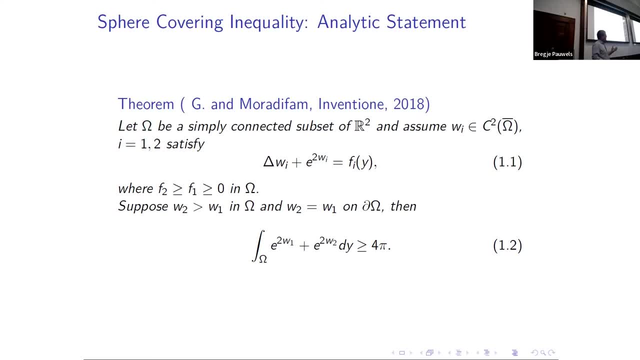 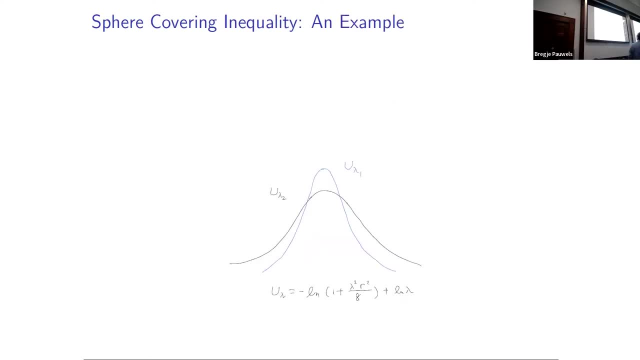 Then why this inequality is true. I mean, it sounds a little bit strange at the beginning. Then I'll just give you an example which may give you an idea why this could be true. Imagine that on the sphere we consider a spherical cap. 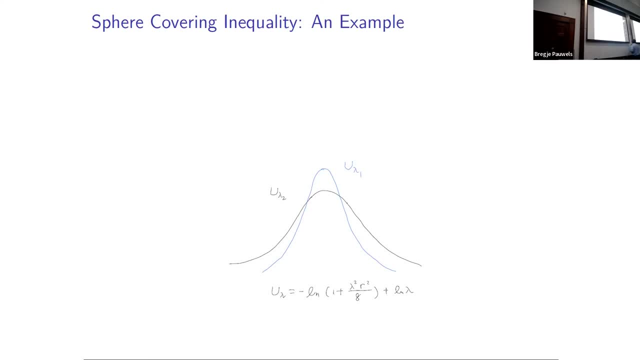 So then we have two right: One is the smaller one, The other one is the bigger one. So we have this same plane to cut the sphere, We get two spherical caps, And if we depend on where we cut this sphere, 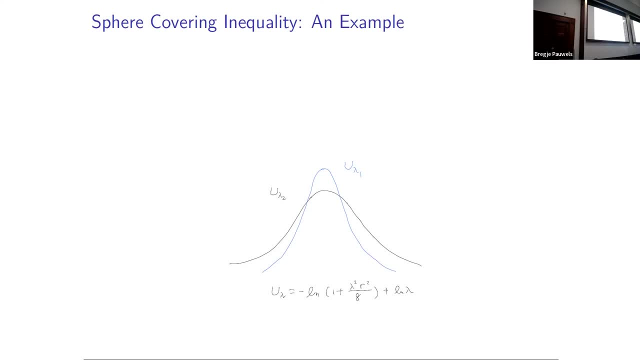 So one cap could be very small, have very small area, The other one will get bigger And indeed both can be regarded as mapping from a disk in the Euclidean space And they have the same stretching on the boundary Where the two caps meet. 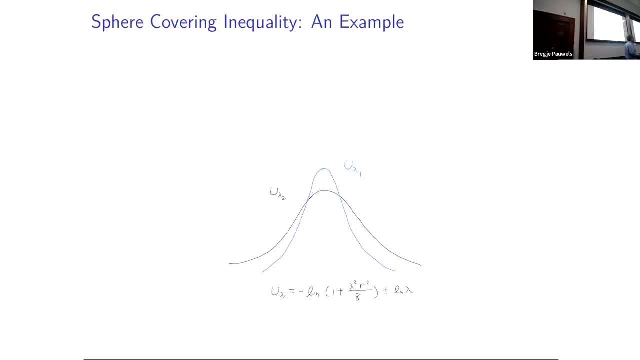 So in this case you have exactly 4 pi as the sum of these two. you know spherical caps Analytically, it is just this simple fact, calculus fact that they are a family of solutions to the Nouveau equation I just mentioned before. 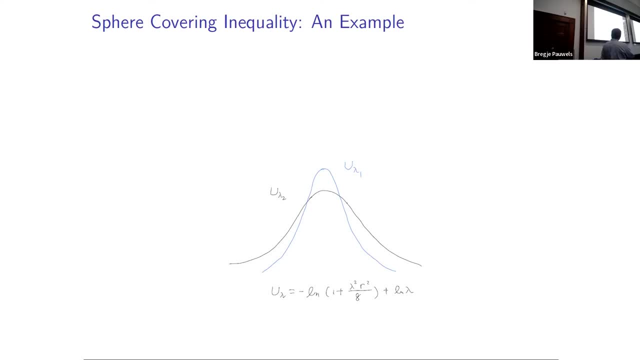 when the right hand side is zero is homogeneous, And then you take two of them, they will intersect once. My picture is not very good, but you imagine that you know. basically, you know bell shape, right, The different bell. 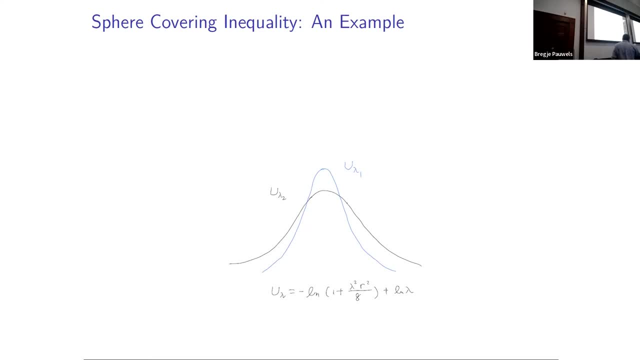 So they will intersect on a circle, And then on the boundary of this disk or the circle, or on the circle they have the same value, But inside they're different. Then to calculate the area of the corresponding patch. 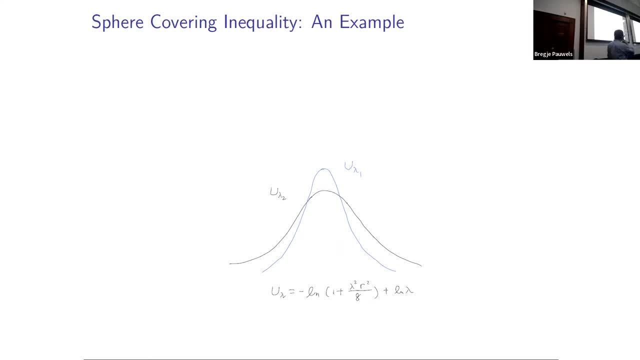 or region is just calculate the integral of e to the 2 u lambda right on this disk. And it's a calculus fact that the area is exactly 4 pi which, of course, geometrically corresponding to the conformal factor. 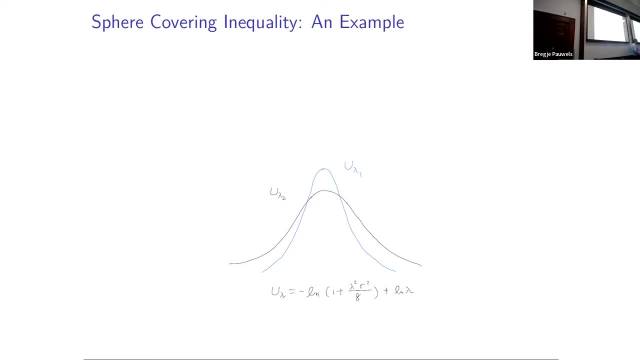 of each of the cap when it's mapped from a disk in a Canadian space. So that's the example, shows that this inequality, you know, makes sense, even though it looks a little bit strange at the beginning. But of course, 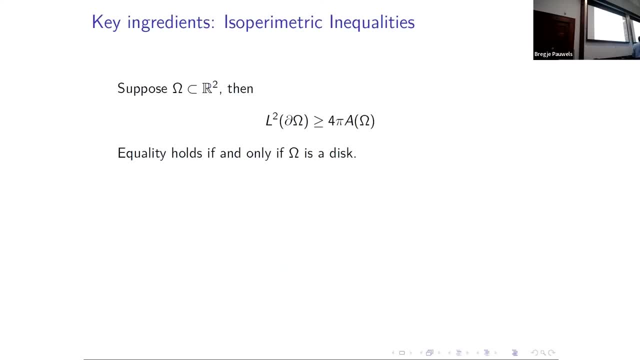 to prove it is much more involved. We have to use isoparametric inequality in various forms, As we know that the classic, the basic, elementary isoparametric inequality says that if you have a region on a Canadian space, then the area 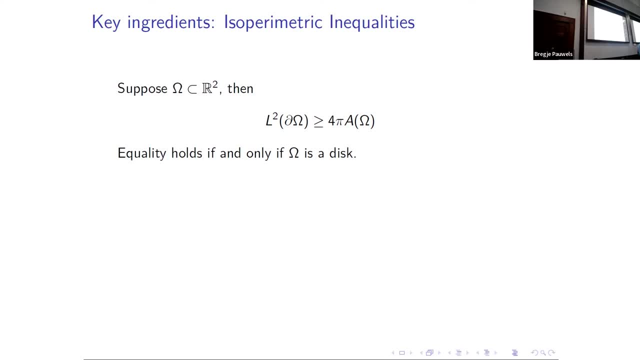 can be controlled by its parameter. So, to be more precise, the parameter squared is bigger than or equal to 4 pi times the area right, And the equality only happens when the disk or when the region is a disk And 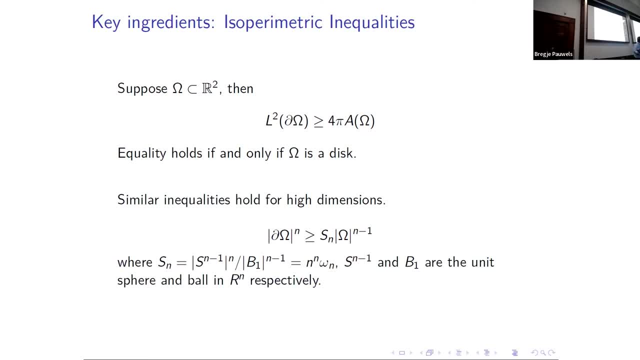 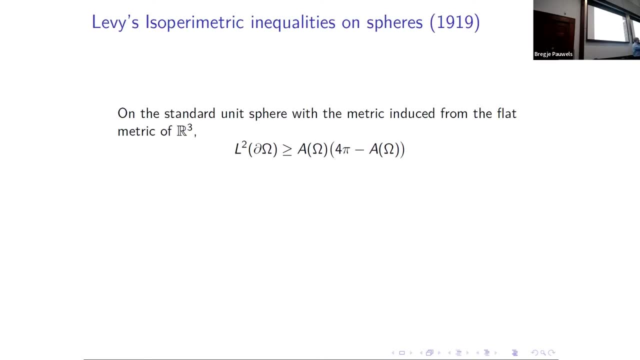 we have also how the mean, or the mean or counterpart, And indeed if we consider a sphere, not a Canadian domain, then we have a slightly different isoparametric inequality. Basically, we have to subtract this term If we do not have. 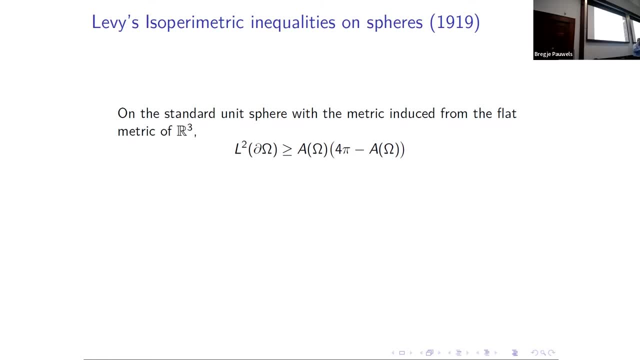 this term in the formula. that's the exact same Canadian isoparametric inequality. Indeed, this is because the surface, the sphere, has curvature. The curvature here is one, So that's the correction term. For example, if we have: 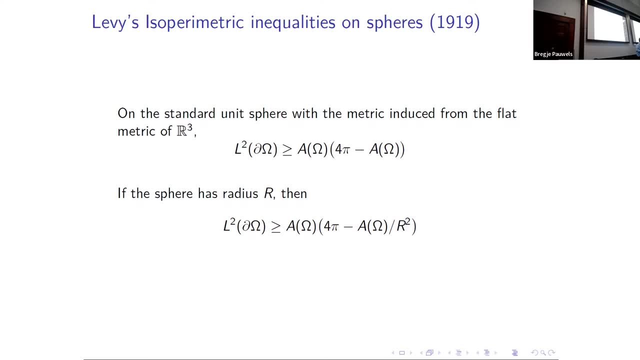 a sphere of radius r. a bigger radius and a smaller curvature, then the isoparametric inequality will have a factor of one over r in front of the correction term. So when r goes to infinity, the sphere becomes a Canadian space. 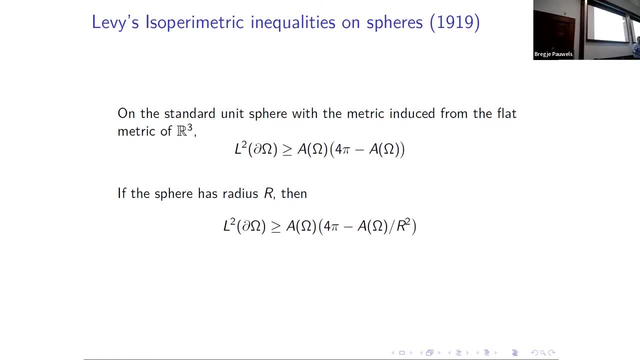 and that factor disappears. Okay, Then a more general isoparametric inequality involving surface is the so-called Alexandrov-Bosch inequality, which has a more general surface, which say we can always conformally map it to a leading 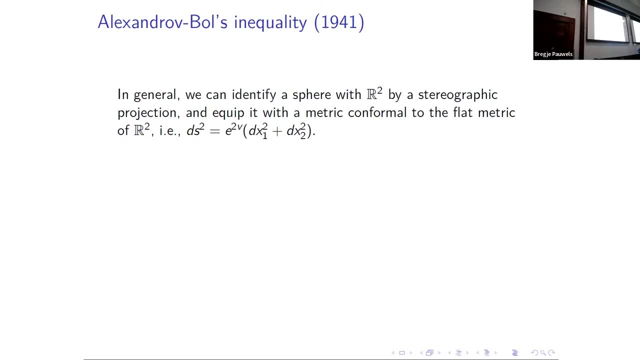 region, So with a conformal factor into the v or function. Then suppose the curvature of the surface is Gaussian, curvature is less than or equal to one which is surface curvature of a unit sphere, Then I mean: 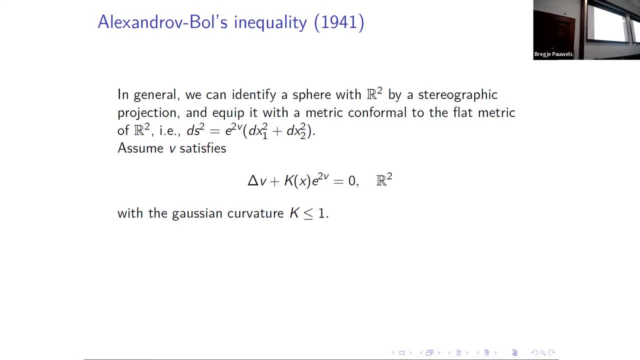 this v, we know the so-called Gaussian curvature equation. So this k is the curvature of the surface, v is the conformal factor. Okay, Then we have this Alexandrov-Bosch inequality, which is as this: Well, 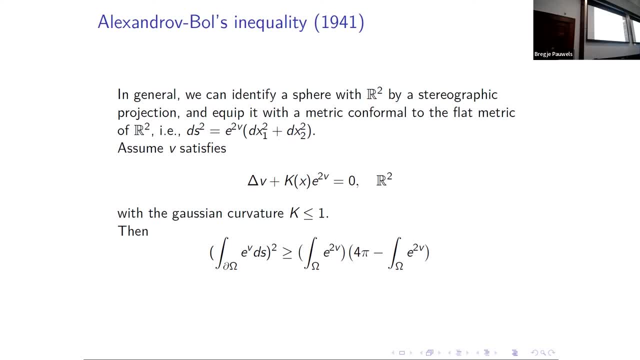 this is parametric inequality, indeed, Because the left-hand side is just the boundary of the boundary with respect to this metric or metric of the surface, And then this is the area of the surface, area of the metric, with metric electrics And this. 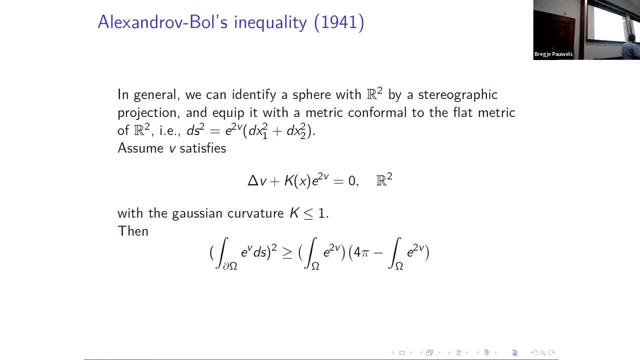 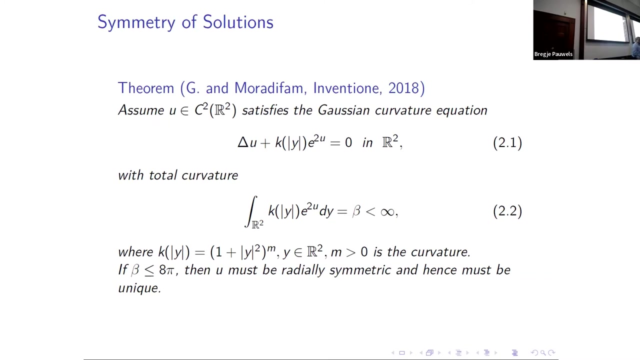 of course, is the correction term, And this turns out to be a very important and useful for proving our sphere current inequality. I'm not here to give the detailed proof, but mainly it's based on this various parametric inequality and rearrangement a technique. 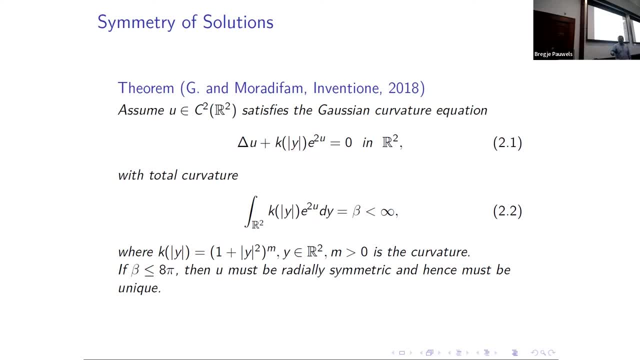 very helpful in analysis and partial definition of the sphere current inequality. Here I'm mentioning a result on symmetry of solutions for PDEs. So look at the partial definition equation like this: Simple looking non-linear PDE famous in geometry and 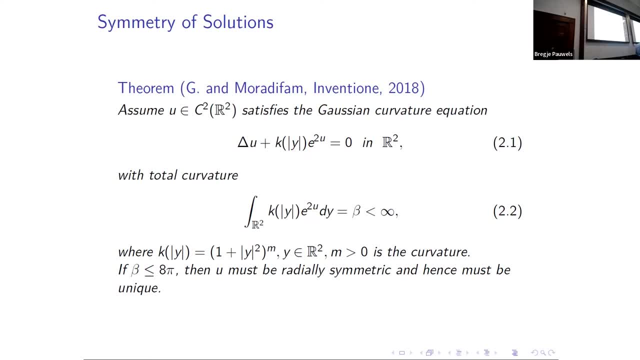 in mathematics, physics And geometrically. it says that can we find a surface which is conformally to R2, but with curve to given as a given function, K? And now suppose K is radially symmetric, depending on only the distance to the origin. 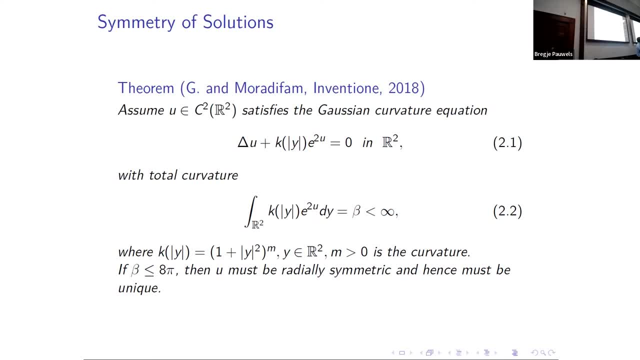 A typical question will be: will the solution U depends only on the radius? Will it be radially symmetric? And this is a very typical question in partial differential equations to prove the symmetry of certain solutions, And this will play an important role in the 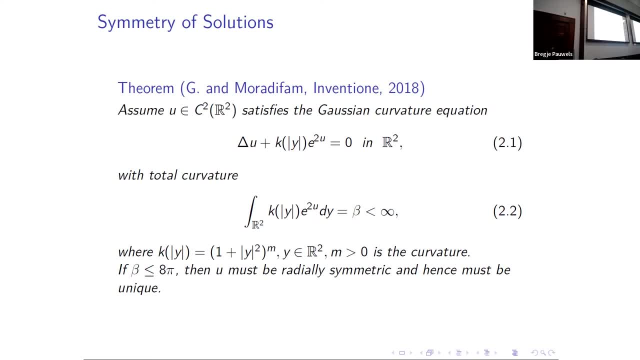 classification of many problems, you know on PDE solutions. So actually can we say the solution is radially symmetric? In PDE area there is a famous method called the move-in play method, which is a very sophisticated way of using. 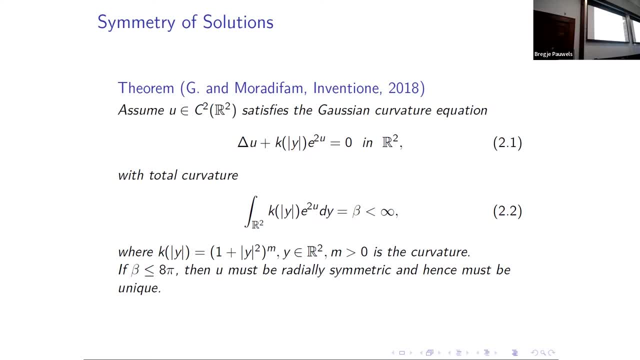 maximum principle of symmetry. Unfortunately, it does not work for this case if K is increasing in the radius. So, for example, K is in exactly this form, but M is positive. the move-in play method does not seem to work. Indeed, 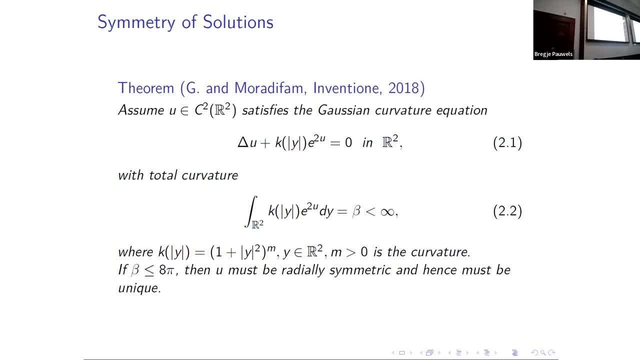 the result of symmetry may not work if there are no other constraints Here. the other constraint we are talking about here is the total curvature. So this integral we usually call the total curvature, and the result is that if the total curvature is smaller, 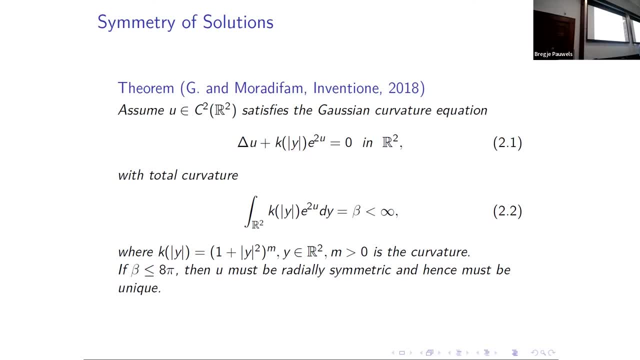 than eta. the total curvature is one. The total curvature is four pi. But here, suppose beta is less than eta pi. we show that the solution must be regionally symmetric, But we mean that it's bigger than eta pi. The answer: 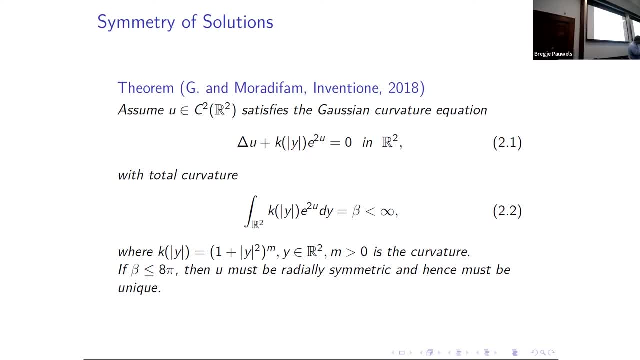 I mean, is not true anymore. There are examples. and to prove this symmetry result, we use the sphere covering inequality And you can see, obviously there's some similarity in appearance of the numbers. So this eta pi. 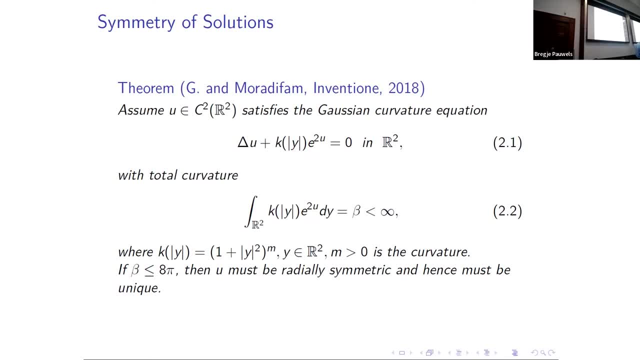 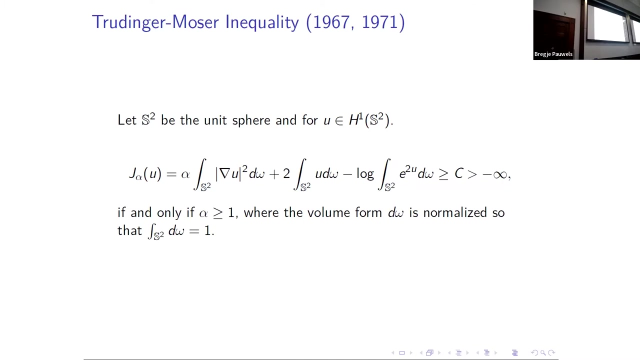 the sphere covering inequality is four pi And you can see that the symmetry is very significant in the study of problems like Moser-Schrodinger inequality. For geometry and the PD, the Schrodinger-Moser inequality is fundamental And 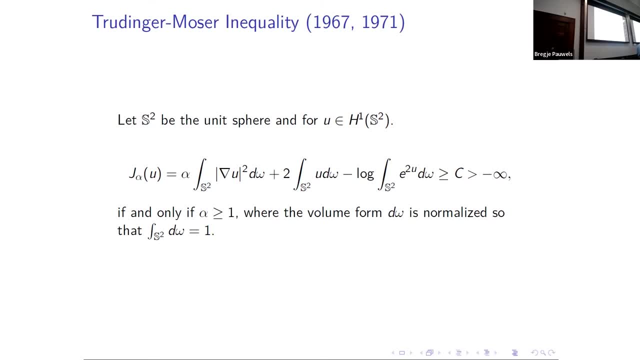 of course Schrodinger-Moser. inequality is an Australian mathematician Everybody knows. And so if we look at the solution u in the superlative space S1,, on the surface, the particular S2,, we 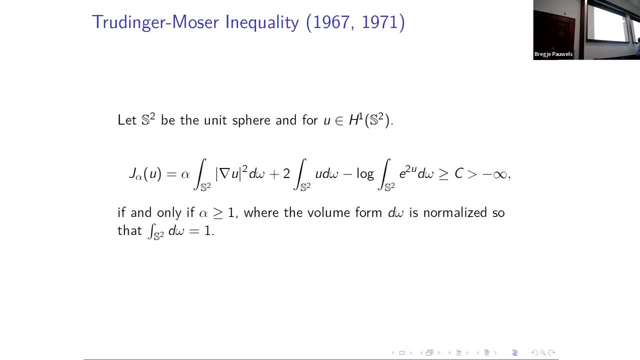 said, the Dirichlet integral will control the Schrodinger-Moser inequality. So you see that, if you remember that in the Schrodinger-Moser inequality the Schrodinger-Moser inequality is very significant And you can see. 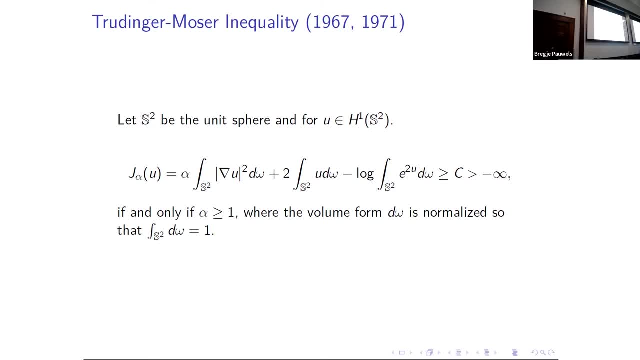 that it is very important to show, Because Trudy-Mozart's inequality says that the integral of e to the 2u can be controlled by the Dirichlet integral of the function. As long as alpha is bigger than or equal to 1, this functional is bounded below. 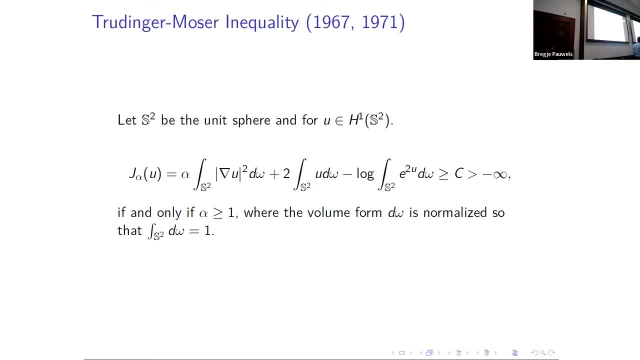 So, in this exact way, control the integral of e to the 2u, And alpha equals. 1 is the so-called based constant, Because if you reduce it by a little bit, the inequality is not true anymore. OK, then a mathematical physicist showed that the low bound 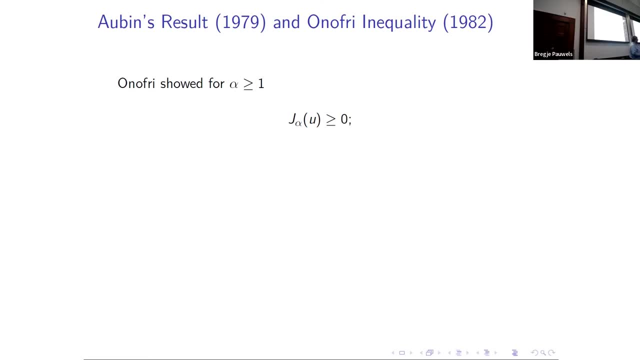 is a constant, So it's actually 0,. very simple and clean. And, on the other hand, if we restrict the function so that its center of mass, which is defined by this integral center of mass is an origin, is fixed. 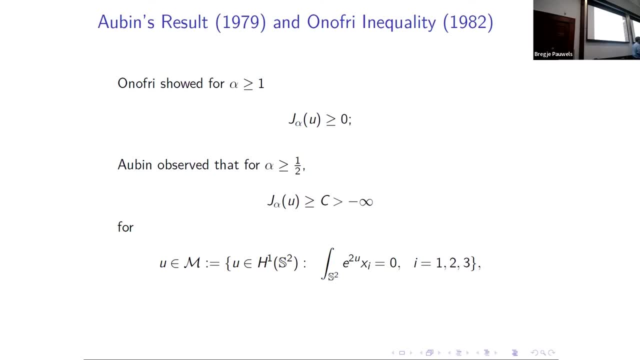 then the basic constant can be reduced by half And so that this functional is still bounded below. So it's not true anymore. And in the 1980s the Gaussian curvature equations, scalar curvature equations, are very popular. It's a hot area of research. 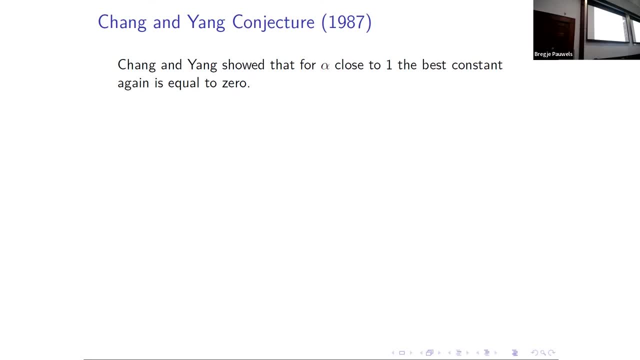 And in the work of Ernest Chang and Paul Yang, they raised the question that whether so the conjecture that when alpha is bigger than or equal to 1, alpha is bigger than 1 half in the constraint set of superlative space. 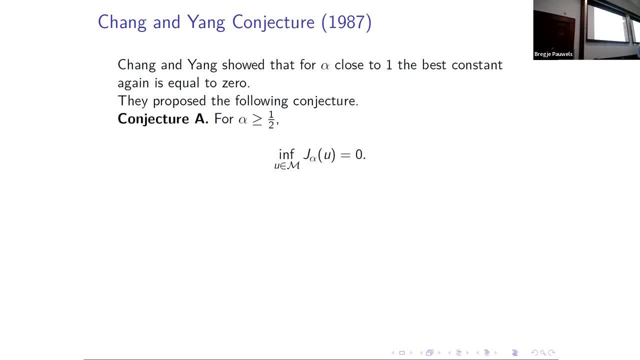 the infimum of the functional is also 0. So, in other words, the base constant can be reduced by half in terms of the- you know, sharp and simple inequalities for that constraint problem. Well, they also showed the evidence why it should be true. 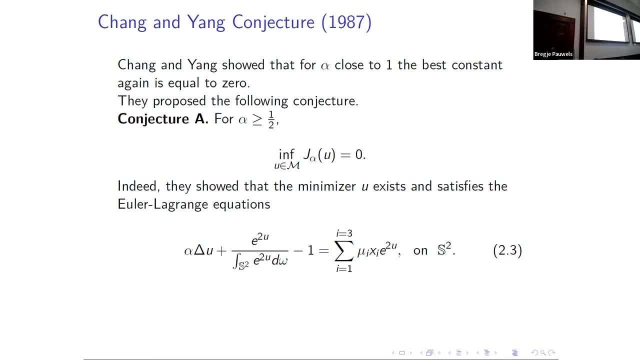 Because for alpha bigger than 1, half the minimizer actually is attained. So then you can find out the Euler Lagrangian equation for the minimizer, which is this type of equation, And indeed there is a mu i, the Lagrangian multiplier, coming from the constraint. 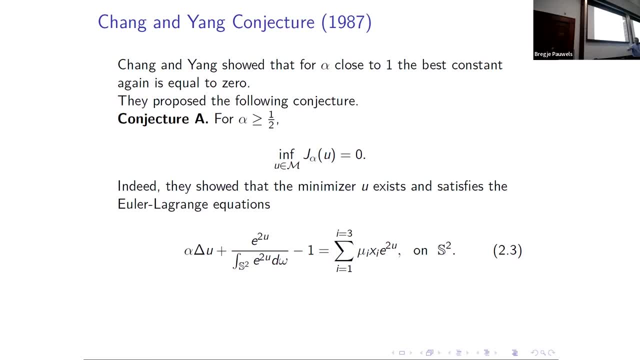 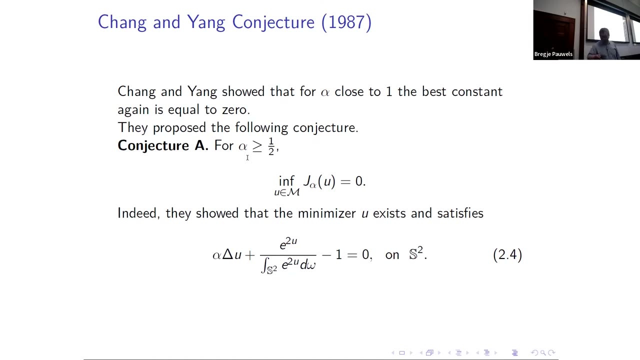 And the center of mass is that origin And this case, and this can be sure that it can be sure that the Lagrangian multiplier must be 0. So the equation is really such a simple looking equation. The right hand side is gone. 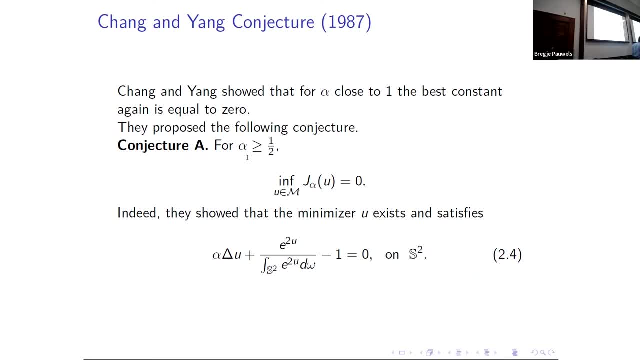 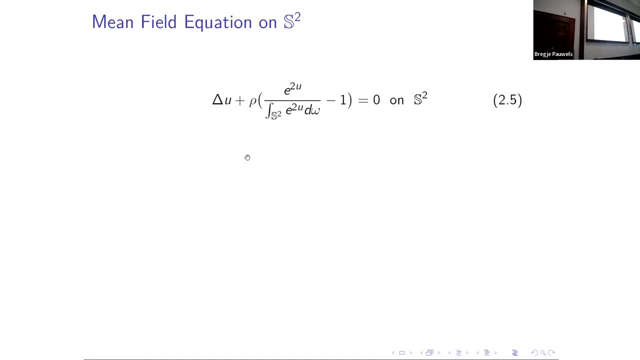 It is 0. So we want to classify or understand the solution for such equation. If we can do that, we understand the minimizer of the function Indeed and, as Chen and Poyang showed, that for alpha very close to 1,. 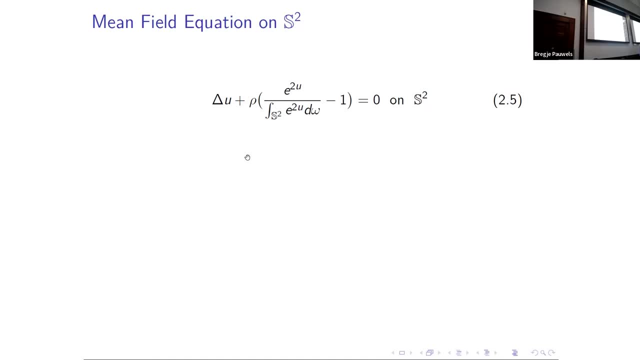 smaller than 1 but close to 1, the solution to the equation must be 0. So, in other words, the inequality must be true. And this type of simple looking equation is indeed not simple at all. It also appears in here: 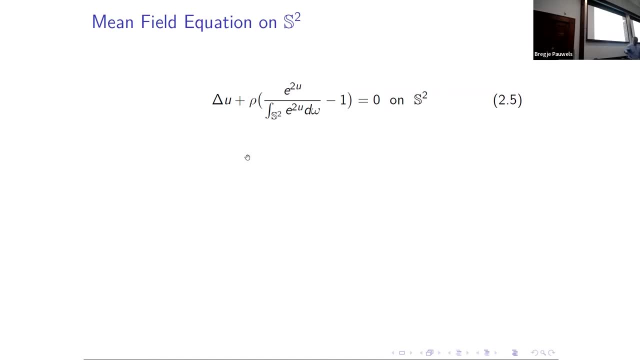 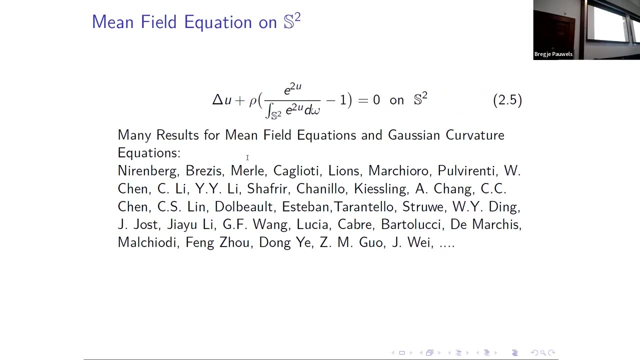 the equation In mathematics, physics, And there are many people, famous mathematicians, working in this area before and now. Here is just a list of mathematicians- Not complete and I may still miss a lot of people. And also this equation appears in the stream: equation: 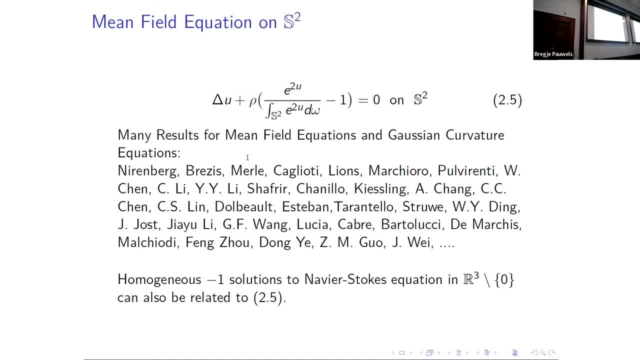 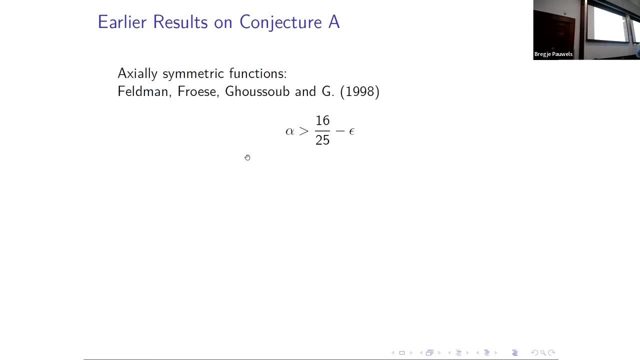 of our Lafayette-Stokes equation for solutions of homogeneous minus 1.. Anyway, I'm not going to go into details. Well, back to the inequality. We first look at the inequality a long time ago, when I was at University of British Columbia. 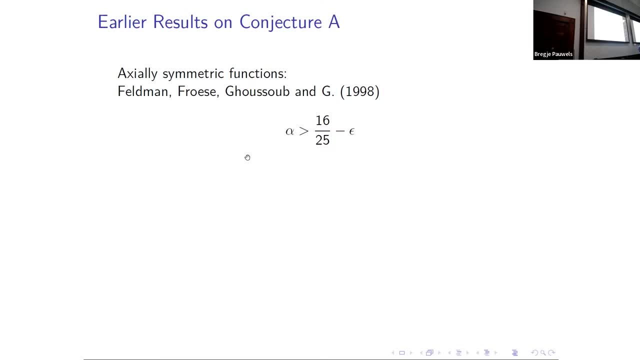 I, you know, my colleagues Ferdman Froese and Nassif Poussou, we know- showed that for actually symmetric functions the alpha can be improved to 16 over 25.. But later this can be improved to half. 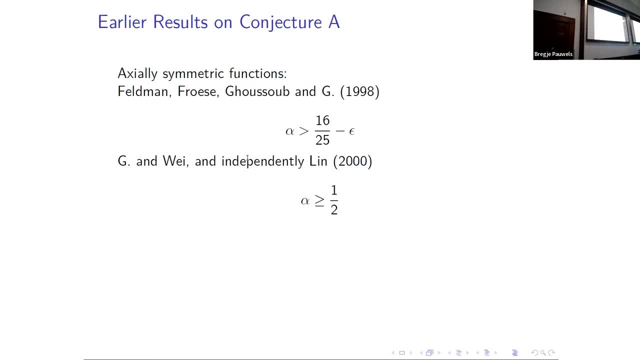 by Junqing Wei and I, and also independently by Changshu Lin from National Taiwan University, And Junqing Wei is at the UBC right now. Later, Nassif Poussou and Changshu Lin: they considered the non-radio case. 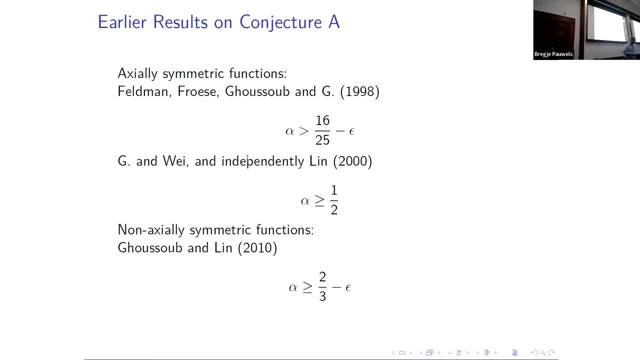 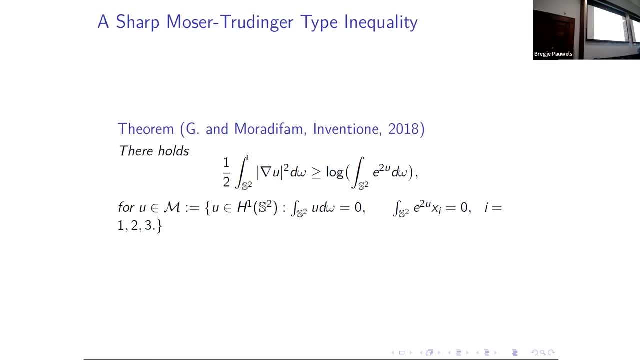 and showed that alpha could be improved to two-thirds. So the latest conclusion result is that indeed, alpha can be improved to one-half, And that's the work for Maldiv and myself a few years ago. So basically, 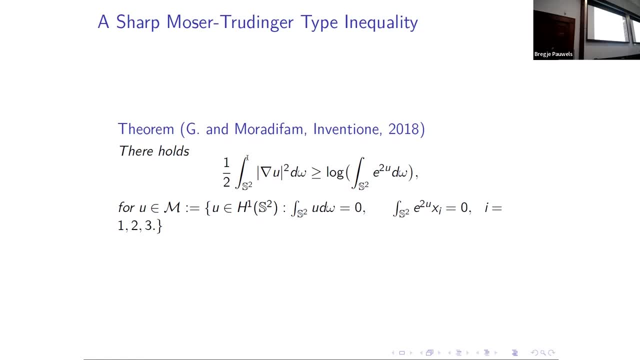 this inequality holds for all functions with center of mass at the origin And the average you can zero. just for convenience, It's not essential. Okay, And to prove such inequality we have the same- I mean obvious strategy. 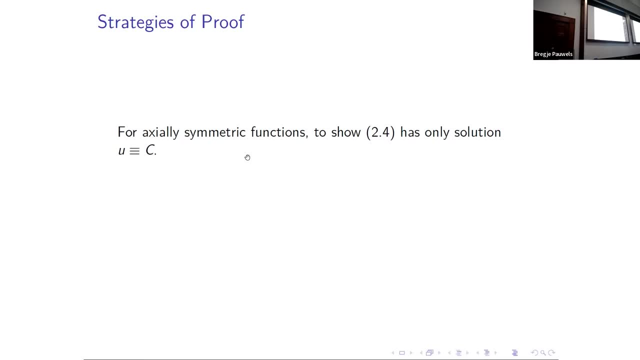 right Because we already showed that for x is symmetric function, the inequality holds And as long as we can show the solution to the PDE, PDE is actually symmetric. we are done Because the minimizer of functional is the solution to the PDE. 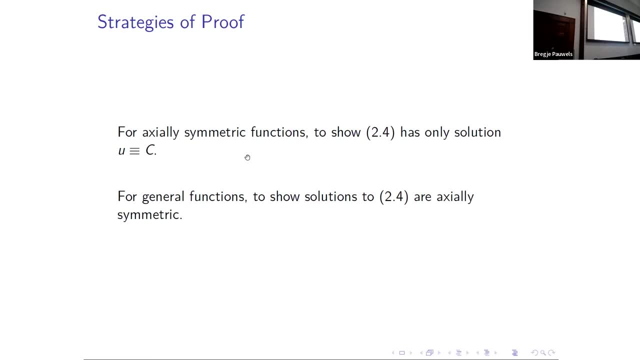 So it might be actually symmetric. Then the minimum is zero, zero. So that's why the symmetry of solutions is very important and significant, And which actually we proved using the sphere carbon inequality And the equation I showed before. 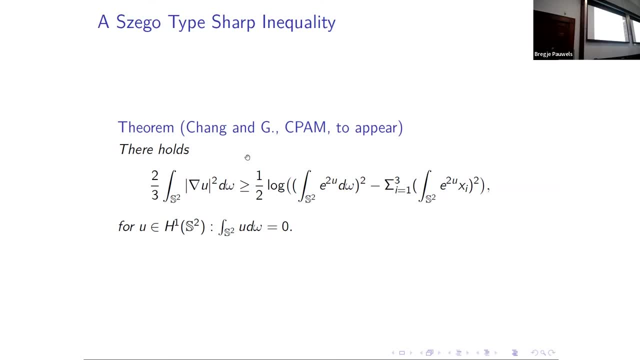 is just a different form of the this midfield equation on the sphere, And I write the equation on the R2, because we have the conformal transformation Anyway. so I'll skip the details of the proof And 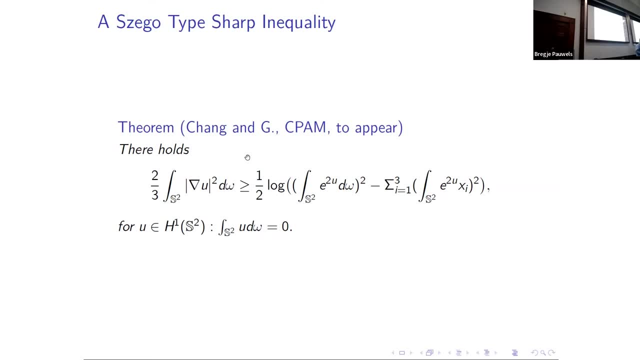 also there are other type of inequality can be proven similarly And in a general quiz we can. we proved the so-called Zeg type: inequality for sphere And well for S1, for circle. 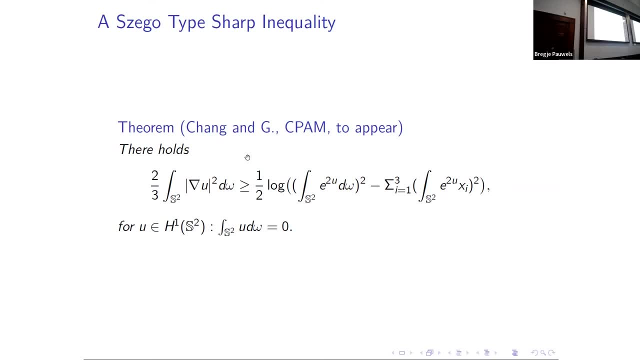 there is a famous sequence of inequalities called the Zeg limiting theory. It is pretty famous in the community of analysis and comparable. So the Zeg limiting theory it is. 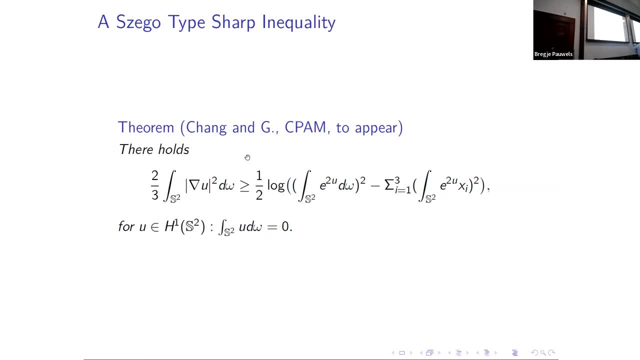 in the community of analysis, complex, particular, complex analysis, And but for sphere do we have simple, similar sequence of inequalities? We showed that at least there is two. The first one: 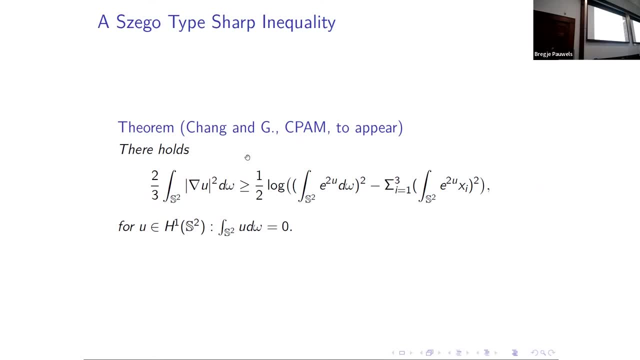 is exactly the Schrodinger-Mozart inequality. The second one which involving the second value of Laplace on the sphere, Which is XI. Okay, So you may. 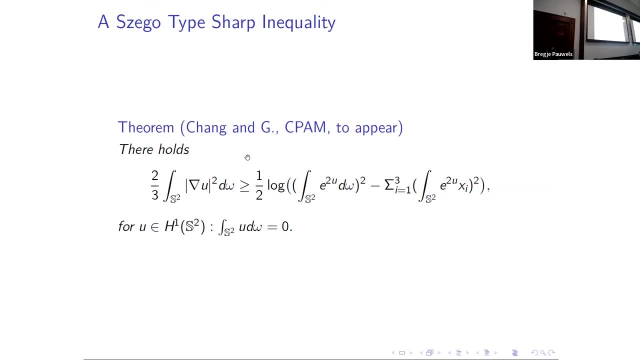 think that this sin of minus of a function is really the coefficient of the expansion of a for the first three functions. So if you 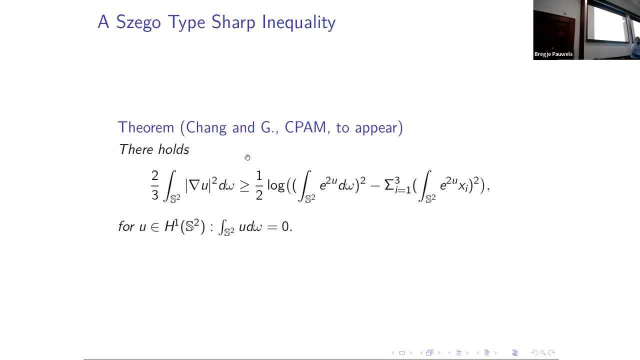 subtract this from the total area, the total integral, can we have inequality similar to equality on S1, which is the, the, the macrame. Okay, 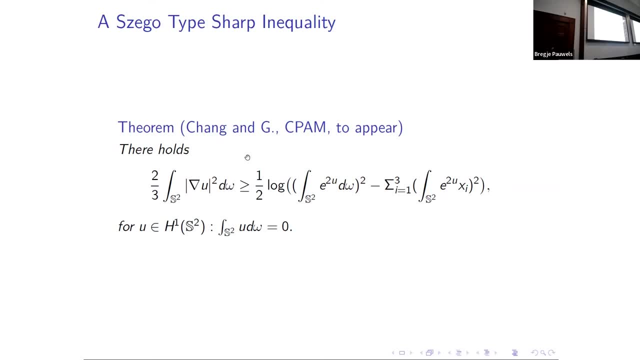 So we have the, the, the, what is S2, So we can. we have a single problem. we can solve the single problem, improve the Moser-Schrödinger model. inequality. 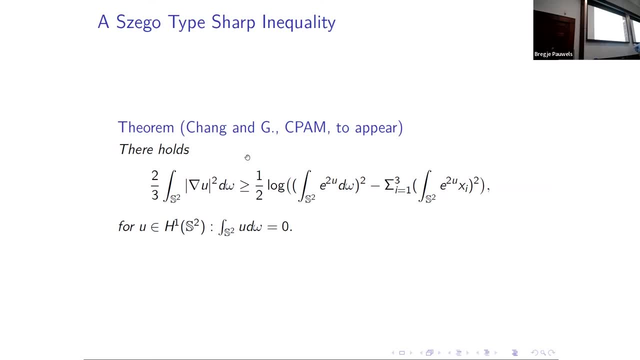 But now, if we put this into the inequality, but without requiring the sin of math to be zero, can we still have one half and the inequality holds? Unfortunately it is not. The answer is actually 2- 3rd. The 2- 3rd is the best constant. 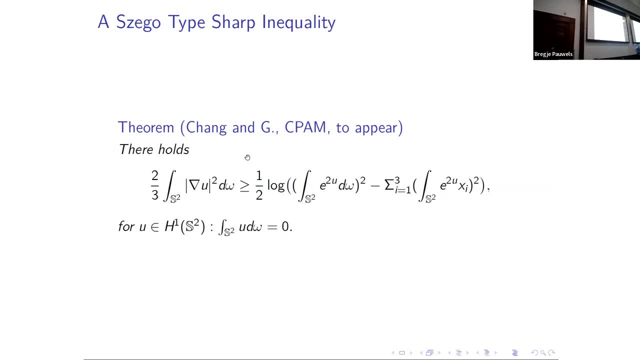 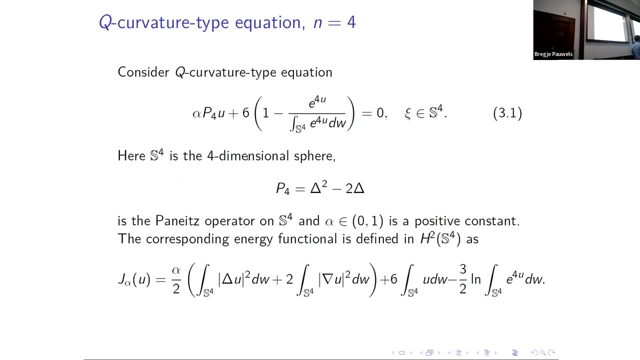 And we show this inequality and also show that if the alpha less than 2, 3rd, it's not true. Okay, So that's the inequality related to Zicke type inequality, And so now we have some sharp inequalities on the sphere. 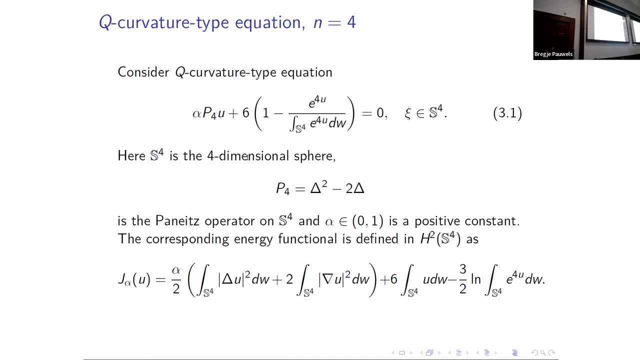 Then how about the higher dimensional space, Let's say sphere? In the setup we can almost do the same thing as we did for 3-dimensional sphere. We can talk about equation, which we call it the high-order mean field equation or Q-curvature type equation. 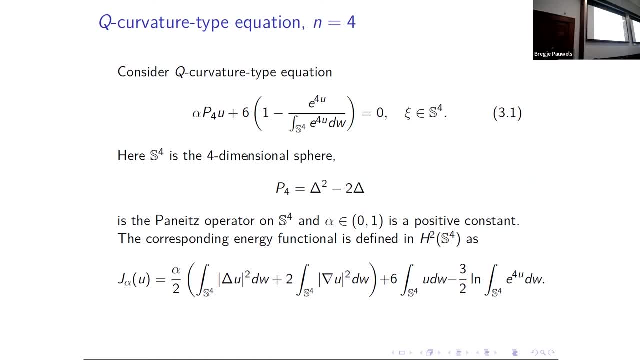 which is exactly the kind of problem we have. It's not part of a mean field equation or Gaussian Q-curvature equation I mentioned before. The difference is that the operator P4 is a fourth-order operator Indeed for S4, it's just Laplacian squared. 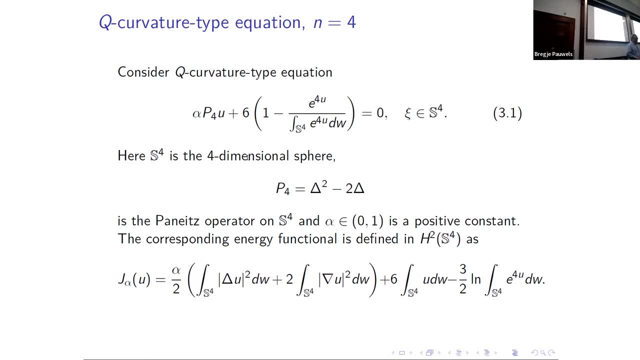 minus 4 Laplacian. We also have this inequality, And indeed this inequality is true for alpha bigger than 1.. And this inequality is true for alpha bigger than 1.. And alpha equals 1 is the best constant, And this is so-called Beckler inequality. 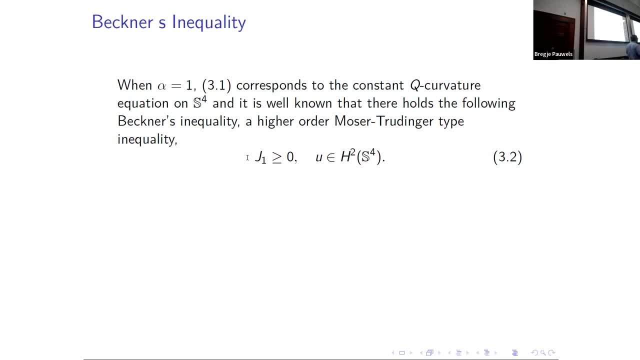 Okay, So a lot of phenomena are similar to S2 in this setup, But because of dimension- right It's a- a lot of difference is expected, Okay, So we would like to ask similar questions. So we would like to ask similar questions. 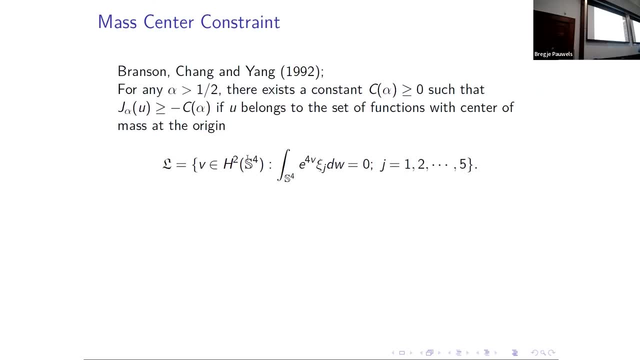 We would like to ask similar questions for the constraint functions. So again, assuming there's a symptom of mass is constrained at origin is constrained at origin origin. can we improve the base constant for s4 in backless inequality? uh, indeed, you know, branson and chan young, they show that if alpha bigger than one half in the constraint setting, 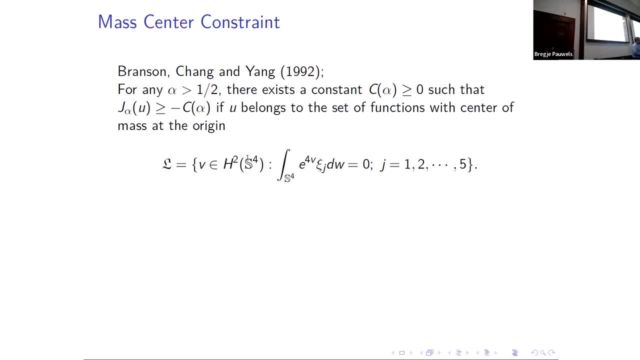 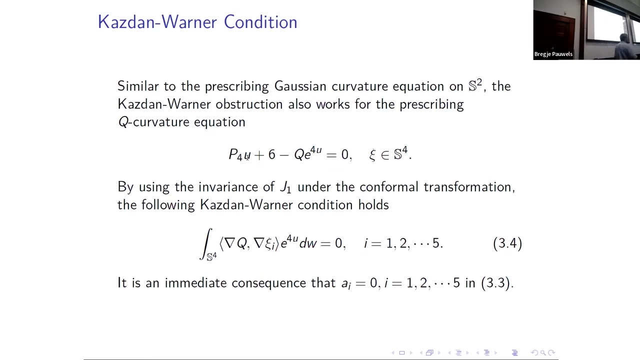 the functional is funny below again, just like in us too. uh, and then you have the minimizer attend and we satisfy the aureola lagrange equation and and this multiplier of uh lagrange multiplayer can also be shown to be zero. and because that's based on the so-called custom warner, uh obstruction or constraint. 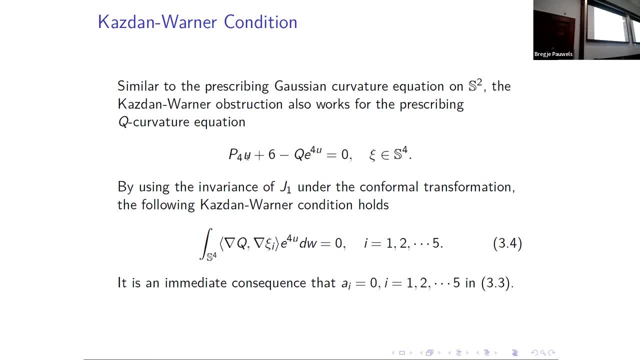 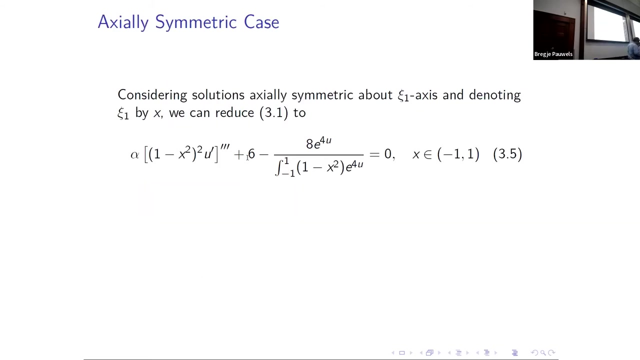 uh which says: if you have a solution to such your opponent's uh operator equation, q is curvature, q curvature- you must have satisfy this equality and this will be used to show that the log runs multiplier is zero. okay, then we want to ask the same question. can be, if you want. 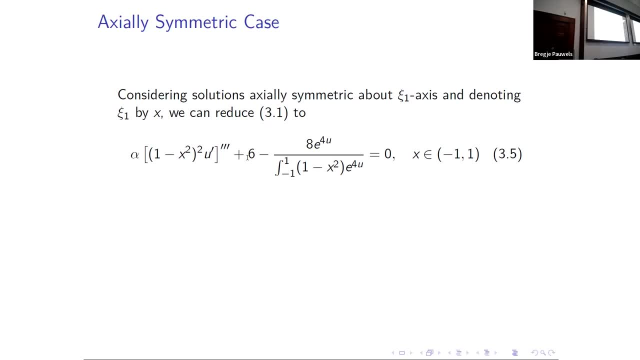 to be zero in the constraint problem. it turns out to be, uh, very difficult, at least so far. we have no way to, no idea how to really solve it. but again, we want to start with the simple case, the function of actually symmetry. so, for actually symmetry, we study the equation, the aureola equation. 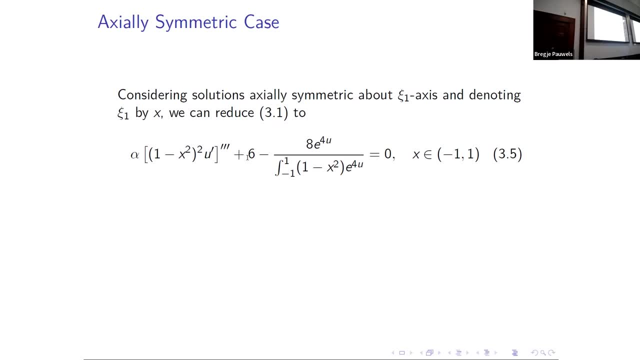 which now becomes an ode, because we have only one variable for the function, which you can say is just the height of the point on the sphere, and s4, but fixed in the north pole and source. so so this is the equation, ode, and of course it's now fourth order equation. and uh. alpha is between: 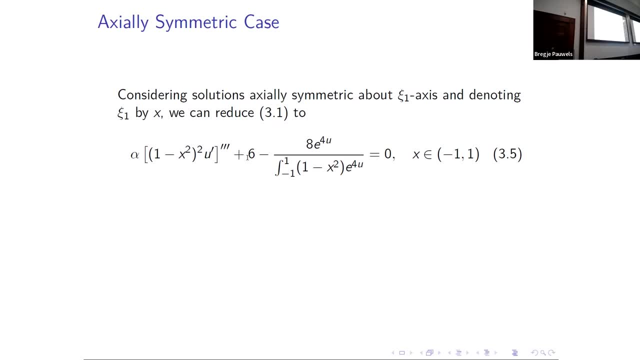 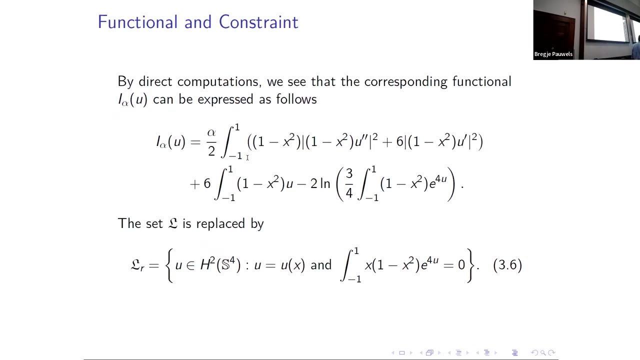 one half and one, can we show that solution must be constant? well, uh, i mean, the equation can also be written in a different way for different purpose, and there's also a corresponding functional. in the simple setting of one variable functions and the center of mass now just becomes such a constraint. 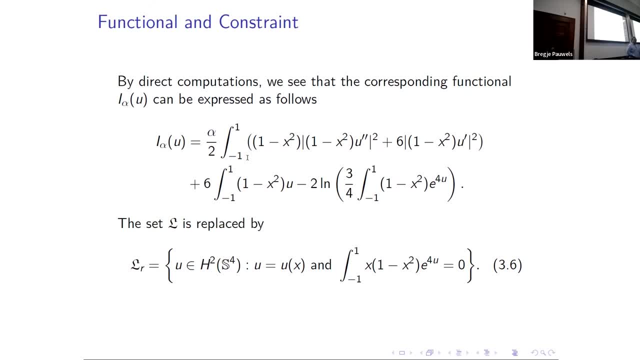 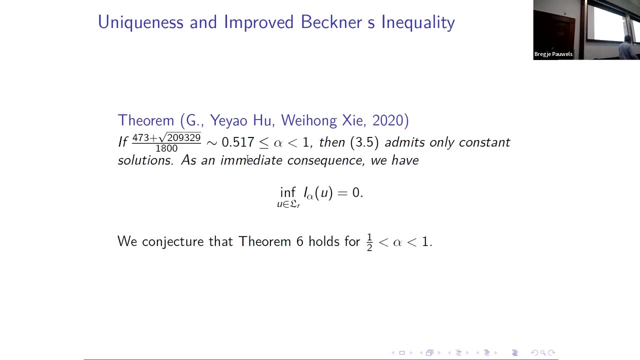 so the, the weight, one minus x squared, comes from the metric of the sphere by, you know, reduced to one dimensional uh interval. well, uh, our result says that. well, we cannot show is true for alpha between one half, but we have a number which is smaller than one and bigger than uh one half. but we can show that this is true and 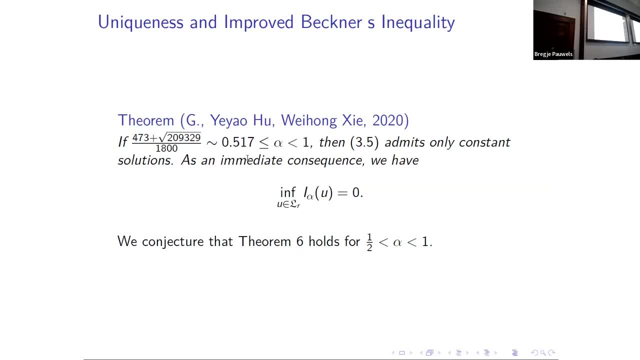 one half. numerically is something like 0.157, 517.. We show that for this range of alpha, the solution I just ODE has only constant solution. So it's trivial basically, And, by the way, this is a general work. 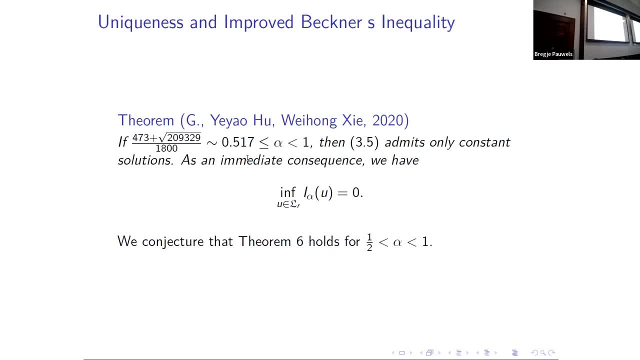 with Ye Yafu and Ye Hongxie, And we did it basically in the early pandemic and Zumi meeting. Anyway, we offer in this range this constant solution for the ODE, and which also means that the etymome in this axisymmetric setting is zero, exactly zero. 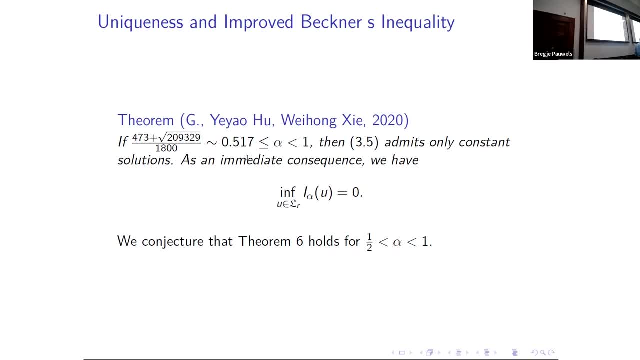 because the minimizer is just constant. The constant make, this function will equal zero. Of course, it's easy to conjecture that alpha should be the best, constant should be one half. Well, from a mathematical beauty point of view, that's what we expect, right. 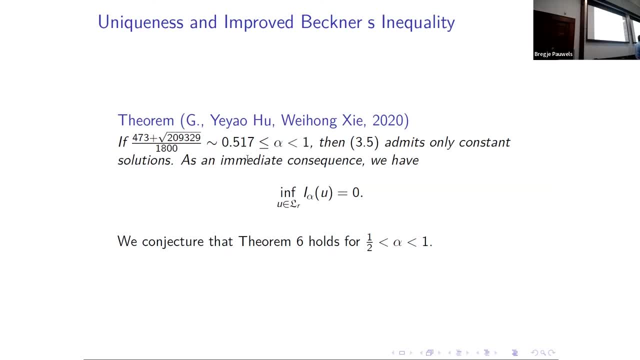 We should expect, But on the other hand, we cannot prove it, And that also make us wonder: would it really be true for higher dimensions? Because the geometry in higher dimensions could be much more complicated, which will affect the result And also analytically. 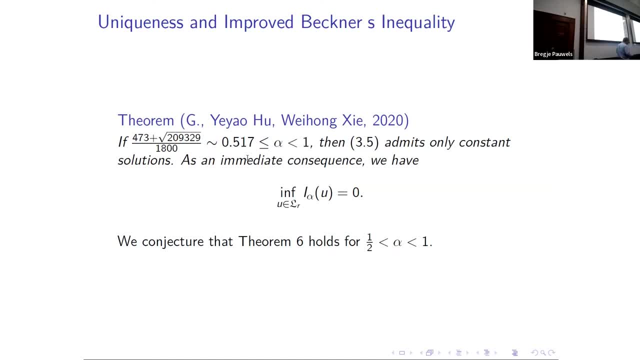 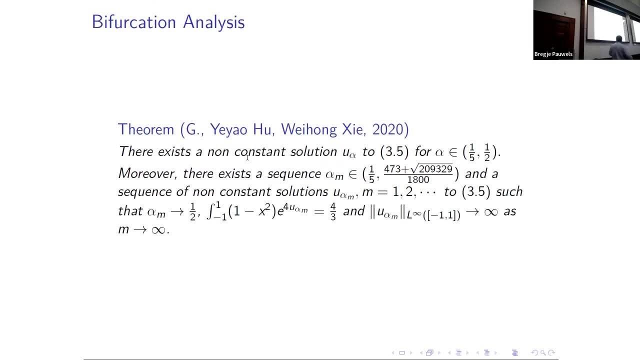 we also have some reservation that maybe alpha is not the best. It may not be the best, okay, Because we also show other. we get some other information of the solution of the ODE. Maybe I show a picture here, So if I show here, 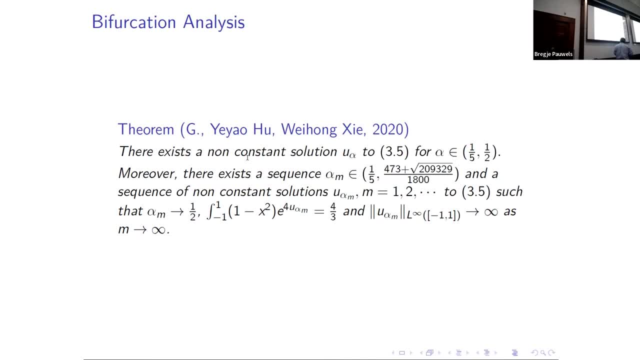 hope the people online can also see it. So if we take one over alpha as a parameter, lambda see- And this picture we see is the solution curve in terms of this lambda parameter, We know when alpha equals one. there's a family of solutions to the ODE. 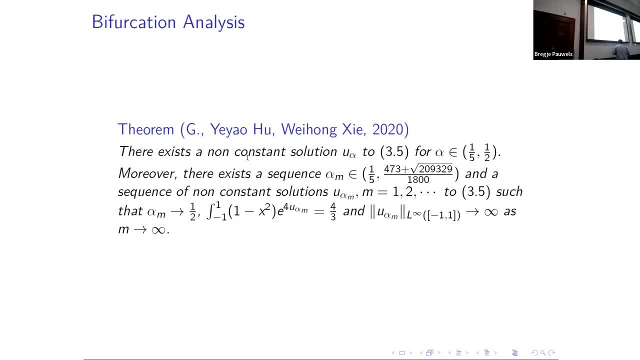 also to the PDE, of course. And then we show also: for lambda equals five or alpha equals one over five, there is only one trivial radial solution. Okay, And there's indeed obfuscation from this. lambda equals five for the ODE equation. 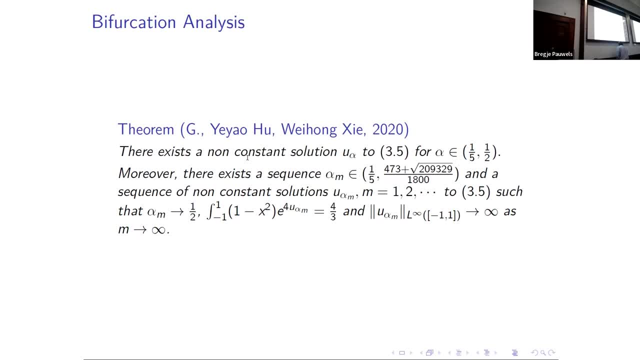 So this lambda equals one. Then we have a lambda equals two, corresponding to the best and the least constant possibly, and we know that the bifurcation of this solution curve. we're not coming back and cross the vertical line here, cross this line here. 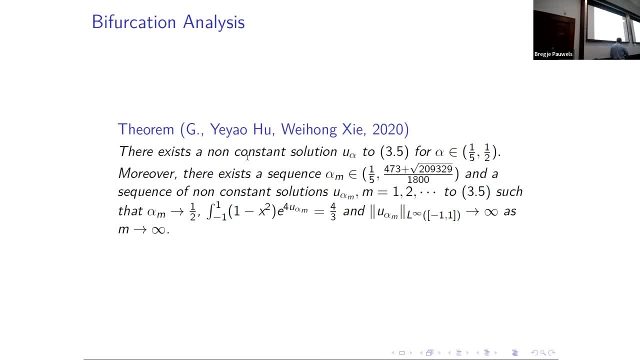 because we show this only trivial solution, So this branch has to eventually blow up. It becomes the more and more trivial solution, So this branch has to eventually blow up, and more and more concentrated on the most power source form And this block point is. a number equals two. 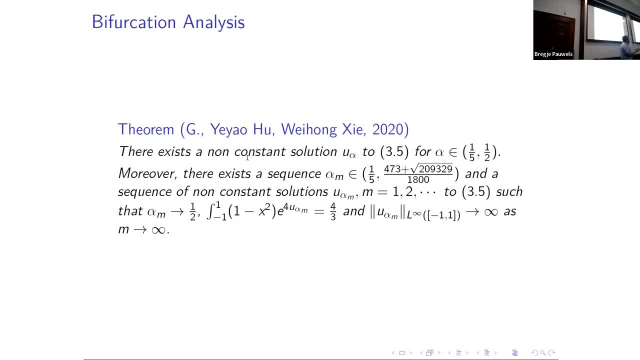 and alpha equals one half And there are a lot of study for this type of block before, So I'm not going to mention, but this is a well known fact. So now, basically, we show that our results shows that this alpha zero 0.517. 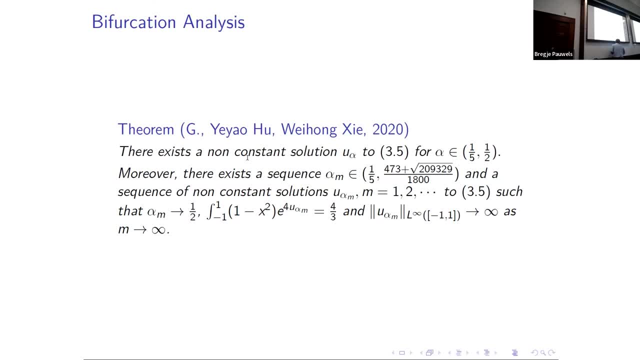 in this range there's only a constant solution, And in this range there's actually non-constant solution. And analytically we do not have a mechanism to prevent the bifurcation branch from crossing this half line. then return back to 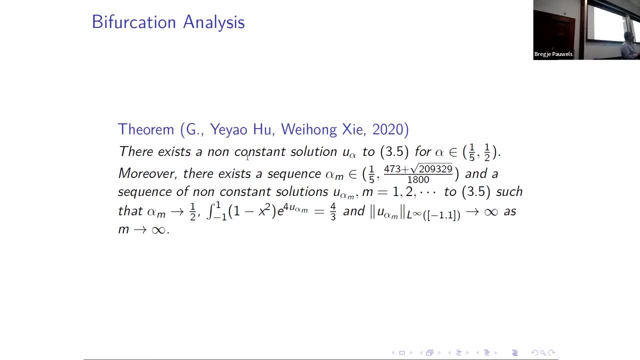 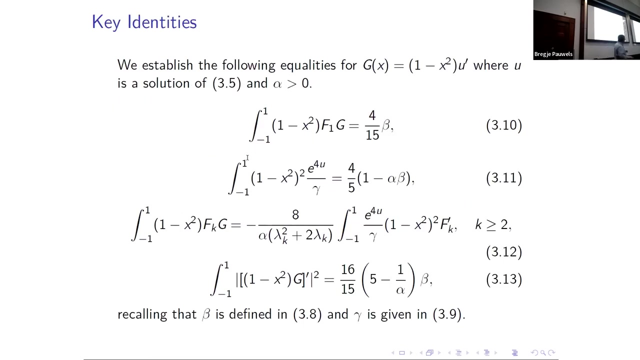 alpha bigger than one half or smaller than one half. So if this happens, of course we cannot get one half as the base constant. So, but this is still open. We don't know for sure And this, as I said, the theorem I just showed. 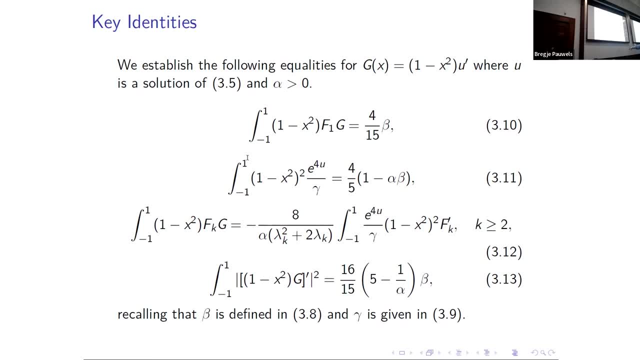 is shown is better than from this picture. Maybe a very quick comment on the proof. The proof analytically is very complicated, So basic idea is that we look at the G- X which is the derivative of U by some weight, multibuffing weight. 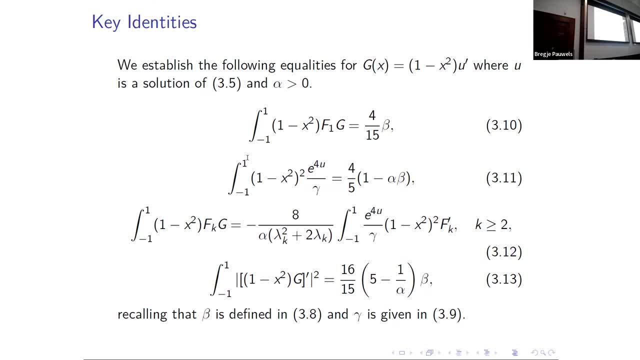 we tried to Have a kind of integrating, if I um, kind of a for real expansion of g in terms of sphere harmonics and the shield coefficients are zero, even, and of course we have non-linear equation. how to use freer type of analysis. 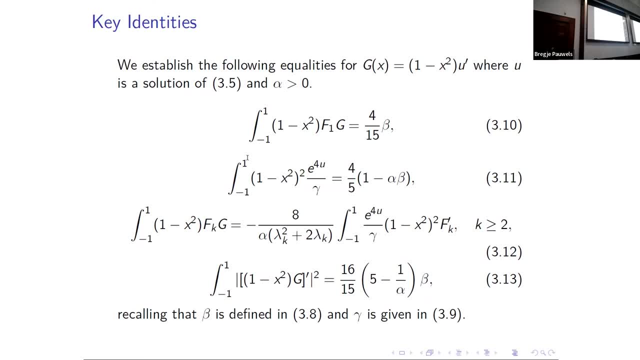 is, you know, non-trivial at all. i mean, usually for linear theory, free series is very helpful, but for non-linear theory, much more complicated. so we have to use a lot of inequalities involving, you know, free expansion- it's more generalist sense, but also we have to use many inequalities. so, uh, one key inequality is that 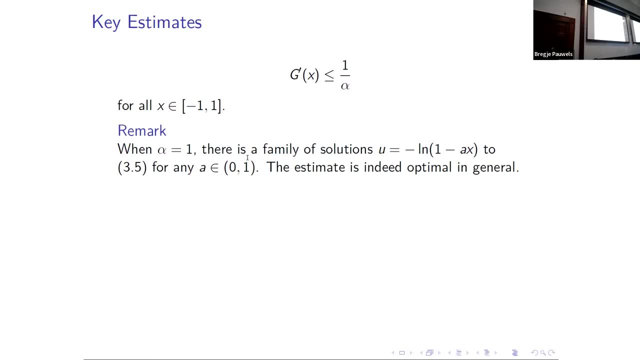 g prime is bigger than it's less than one half for solutions of this equation, and i don't know what's the geometric meaning of such inequality. and that's what we proved, you know, analytically. so, using this inequality and the equalities, we showed that the g, this special function, can be controlled in this way. 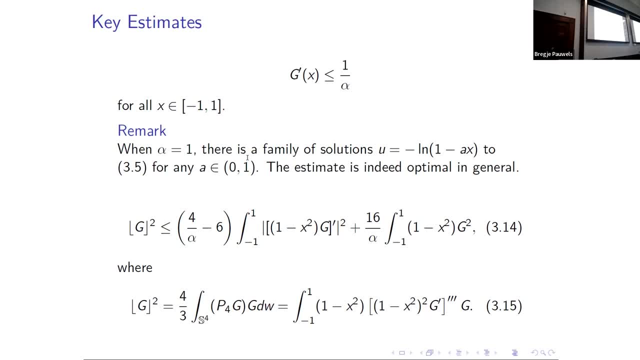 roughly speaking, it says that h2 norm of g can be controlled by h1 and the l2 norm. but we know from pde point of view lower order norm can always control by higher order norm. so h1 and l2 norm can be controlled by h2 norm. and then you have a, you know g h2 norm controlled by constant times: g h2 norm. if 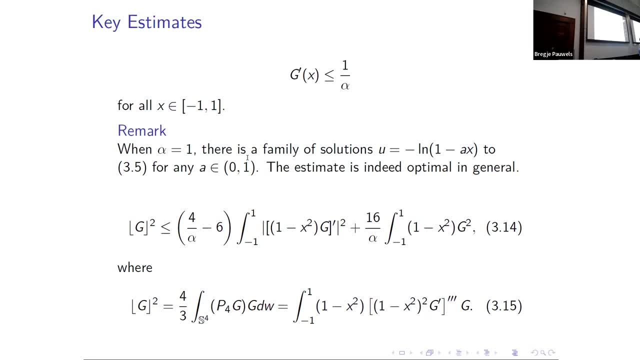 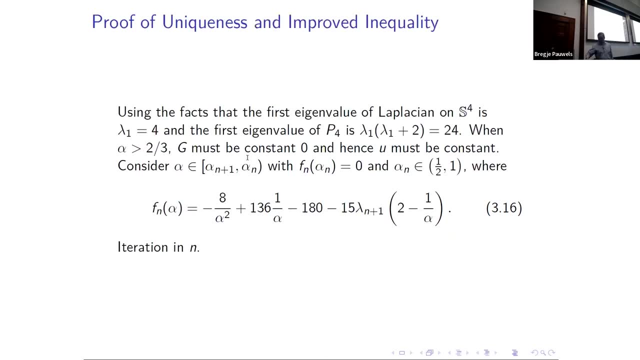 you can show this constant is less than one. you can show this constant is less than one. we can show g, zero. that's exactly what we're doing: um, so uh. but of course, to eventually get the number uh, we have to do iteration. hopefully the iteration even give us one half, but unfortunately 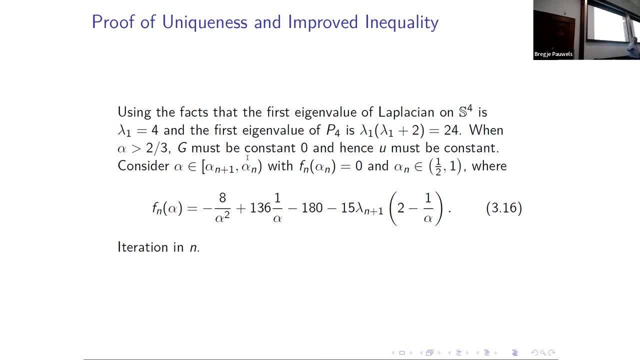 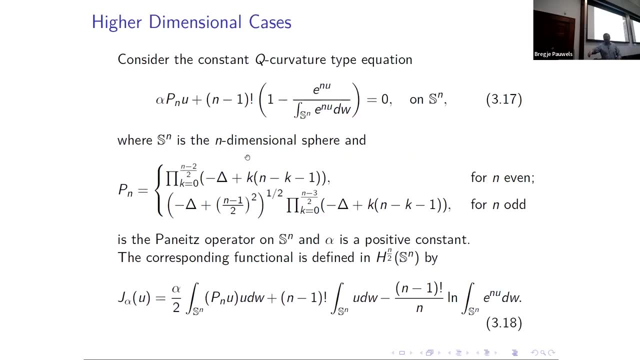 the iteration will stop at some point, uh, some step, and that's what we, why we get that strange number. and now of course we can do the high order, uh, higher dimensional case, like a general 2n dimensions as 2n. they set up again similar, uh, the operator now becomes sort of the penance operator. 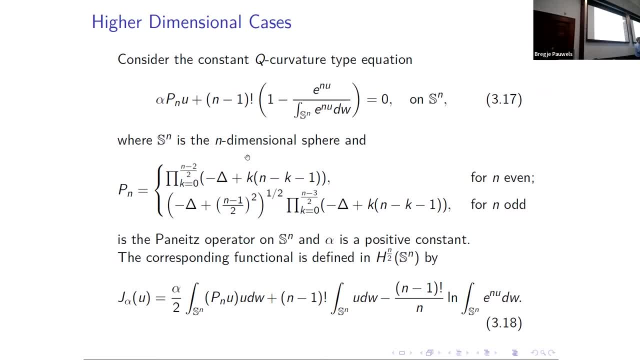 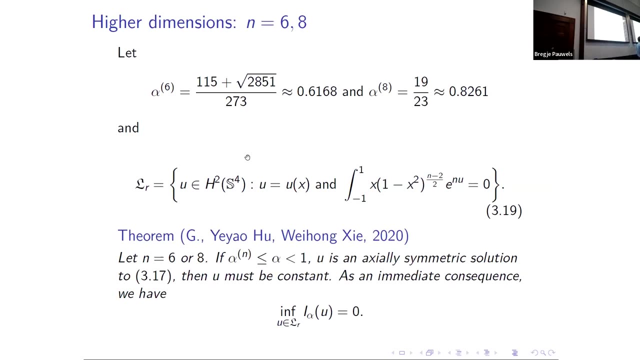 as a pn, which is two n's order differential operator, and we can talk about sphere harmonic functions for such a higher dimension sphere and do it similarly as we do for dimension four. so far we can get a similar result for dimension six and eight, and this two number still less than one, are bigger than one half. 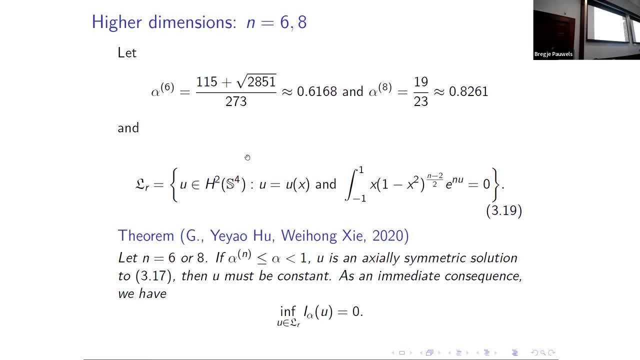 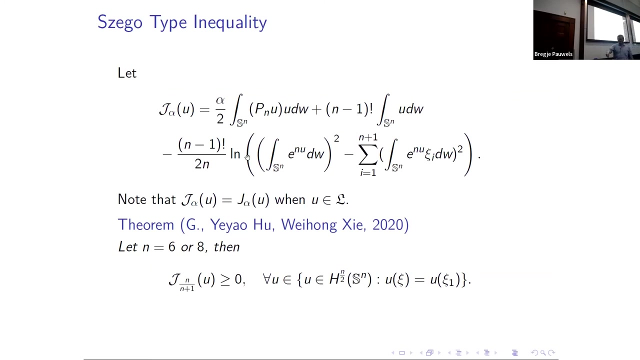 we use our last, but we'll show you the difference in the loss and we show a similar result. okay, and of course we we hope to do it for all the even dimensional space. but there is a calculus, uh, technical difficulty, uh, which, um, i, um, i can just very simply explain. 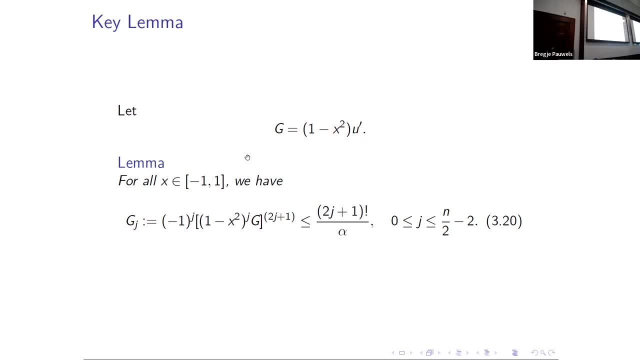 um, so for, um, so for. By the way, we can still get a lot of inequality involving this function G. So we can get higher order differential inequalities with G And then we try to express such an integral in terms of G which we have already shown the inequality. 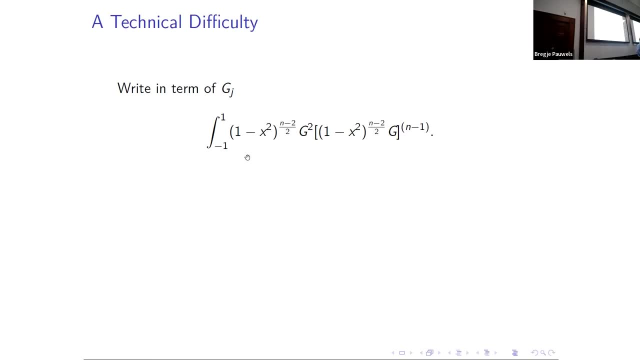 There are many such terms, but you know finite n over 2 terms. We want to express this integral into those special forms. For two dimensions, this term is 0.. For 4,, 6,, 8, we can estimate them just. 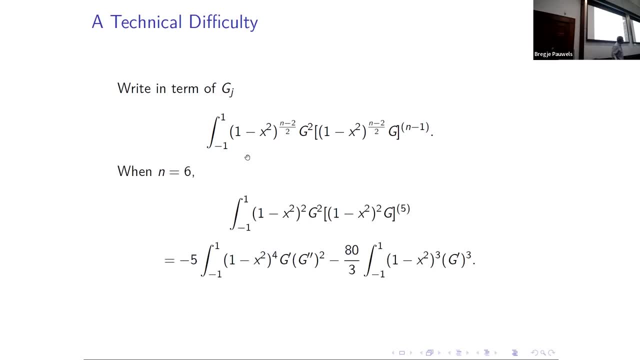 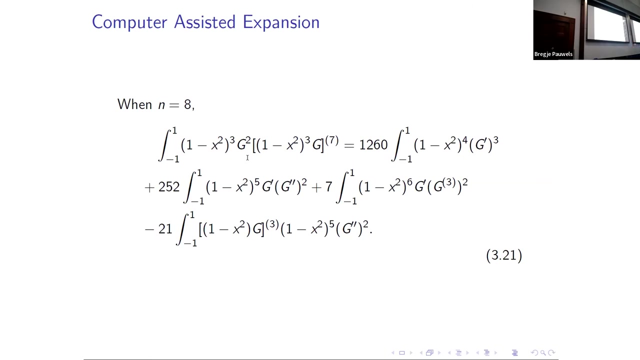 by integrating by parts right Just formulas. For example, for n equal 6, we can have this decomposition. Both terms below can be estimated. And for dimension 8, the expansion gets more complicated. And to do it by hand, it seems. 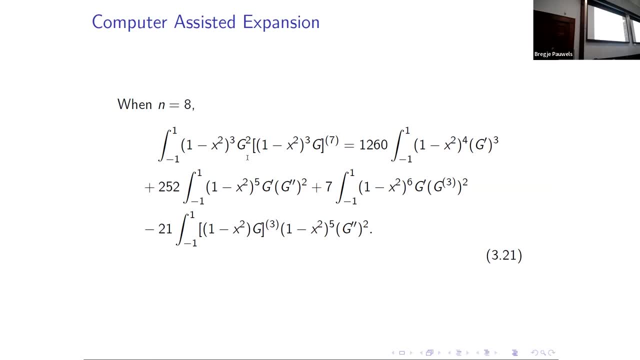 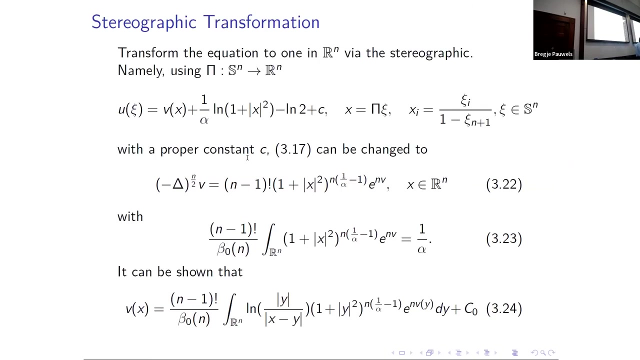 not easy, so we did it by computer to help us to get this formula. But for dimension 10 and higher, we don't know how to make such decomposition, Or we even do not know if there is such a decomposition. Anyway, that's why we do not go to even higher dimensions. 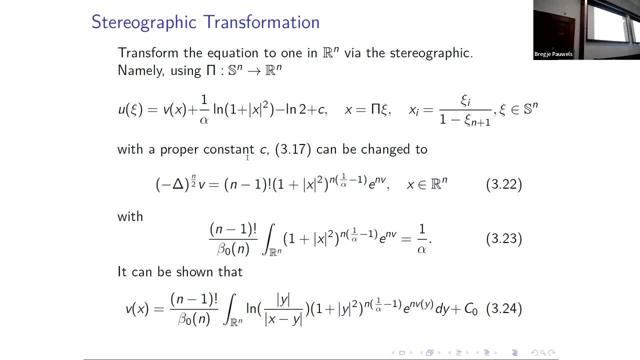 Maybe I don't know. Quickly I will mention: there is another way to study the equation by using the so-called stereographic projection, but change the equation on the sphere to equation on rn, or actually r2n or even dimensions. 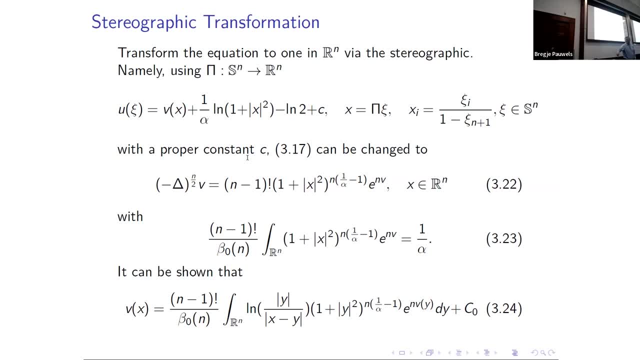 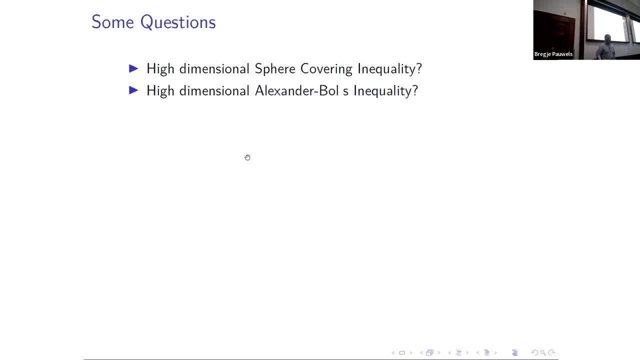 And then we get- because I don't want to get too much time, too technical, So eventually we get the equation which, involving higher order equation on rn, with a coefficient increasing the radius direction, So to solve that problem. so basically this equation okay. 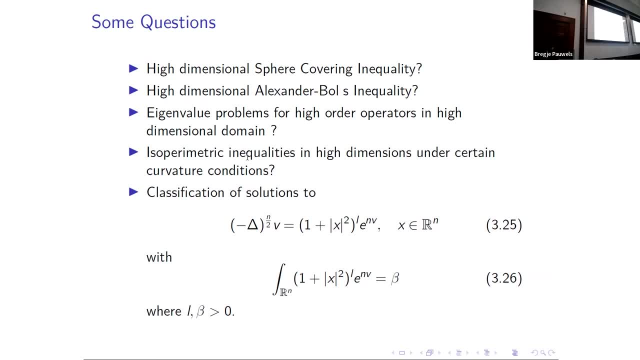 And then we want to classify. But the solution of this equation for l bigger than zero always told the curvature, q-curvature, to be given as a beta. To do that, if we want to follow the same strategy as in two dimensions, we need to show. 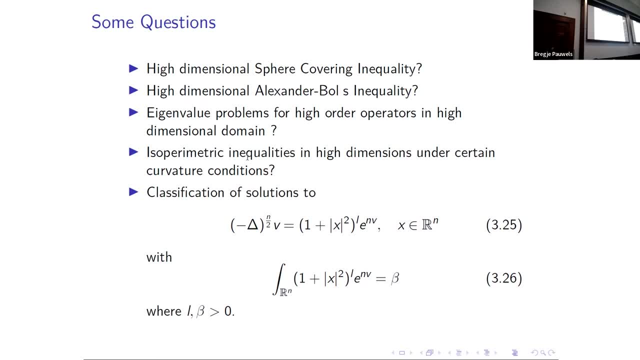 higher dimensional sphere covering inequality, which we'll probably do later. So that's what we're going to do. We probably need the higher order Alexander-Wolf-Boss inequality, higher dimensional, which basically higher order, higher dimensional, as a parametric inequalities. 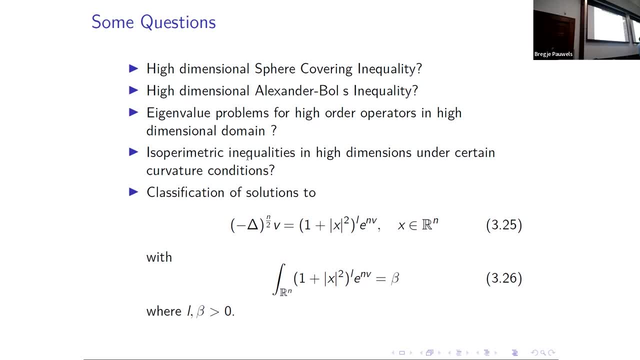 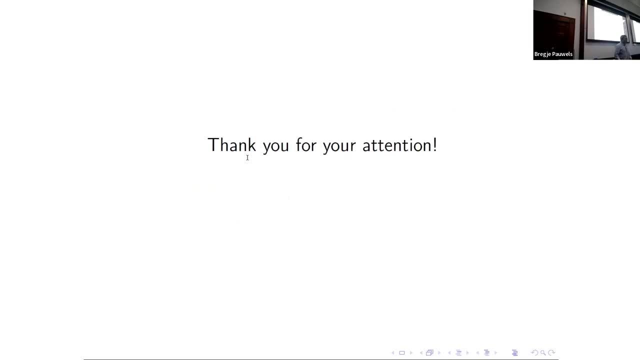 and some weak curvature conditions, And all these are open. So I stop here, Thank you. So I have a question. Yeah, So So we're also looking basically for the sphere governing inequality on S4, is this right? That's right, yeah. 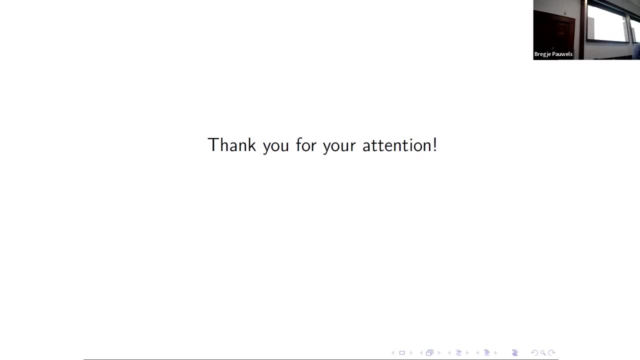 But you could not prove it because, or what was exactly the point? where did you reach it to? Okay, So On S4.. Yeah, For S4, there are two major difficulties. First, there is a parametric inequality for both dimensions and the weak curvature conditions. 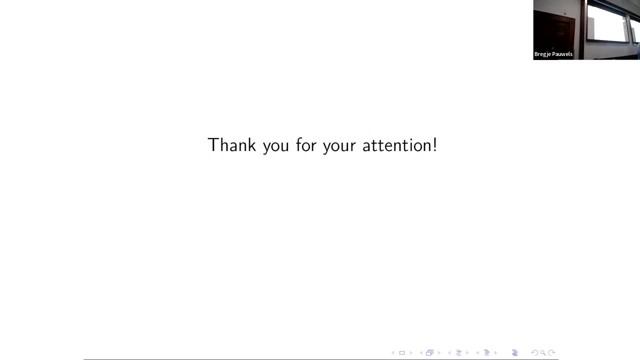 So if you have a strong curvature condition, like a rich curvature has certain, you know, upper bound, then there are some parametric inequalities, like a Gromov or Levy-Gromov inequality, But with weak curvature conditions, for example, just like. 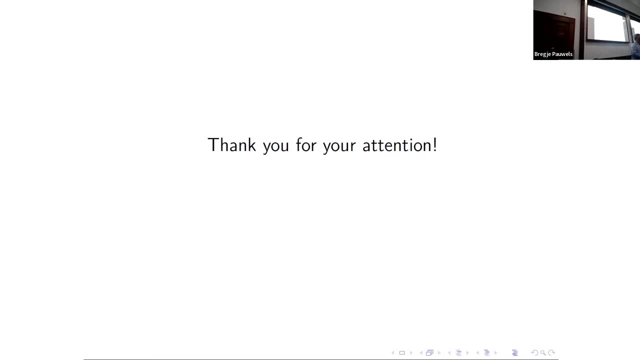 The scalar curvature conditions. do we have, you know, similar simple but sharp as a parametric inequality? I don't know. Secondly, for rearrangement: if we use a rearrangement, the level set, you know, is not good. 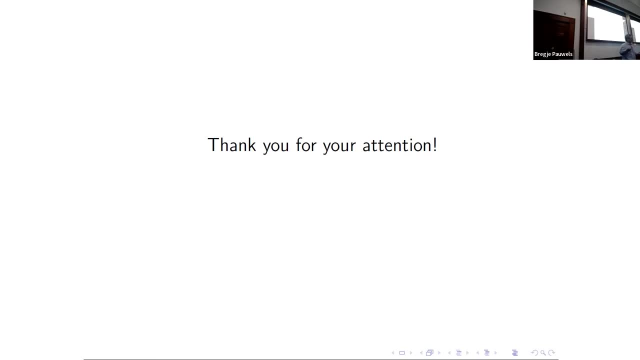 So you know, in R4, we have a three-dimensional surface right, You know, hypersurface, Which is much complicated For two dimensions. the level set is a curve which you know is relatively easier to handle. 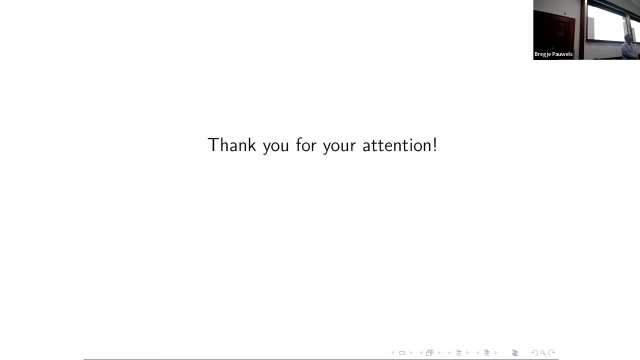 So that's two major difficulties: to show the sphere curve inequalities in higher dimensions, And indeed we do not know if it's true. Okay, So if it's true, what's the right formulation? It's still not clear because of course, eventually it depends on you know the analysis. 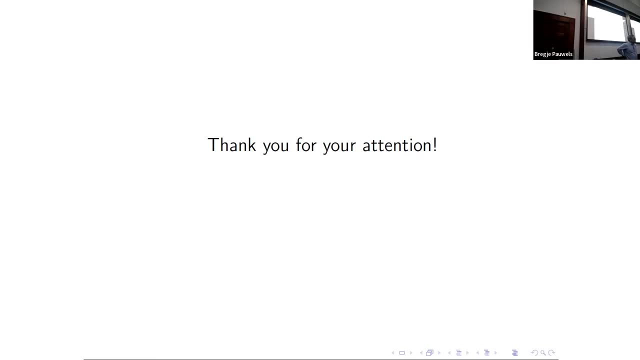 Forget the right form. Thanks for the very good explanation. Very good explanation. Are there other questions? Thank you. Symmetric solvations page in R4.. Yeah, Actually, the counterexample data is given on the 8th power. 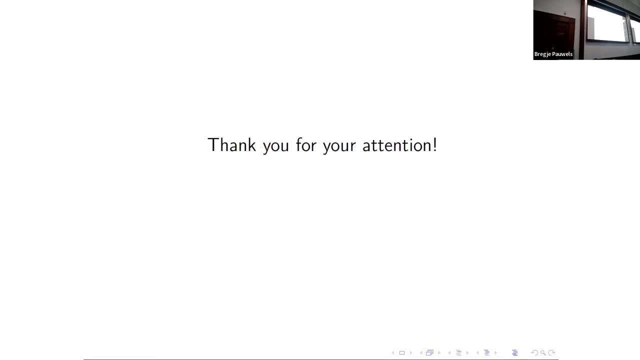 Yeah, Can you give us intuitively? what is that? counterexample, right? How can we explain intuitively? Well, let me take this picture. Okay, We know that for alpha less than 1 higher, there is a non-constant solution for the equation.